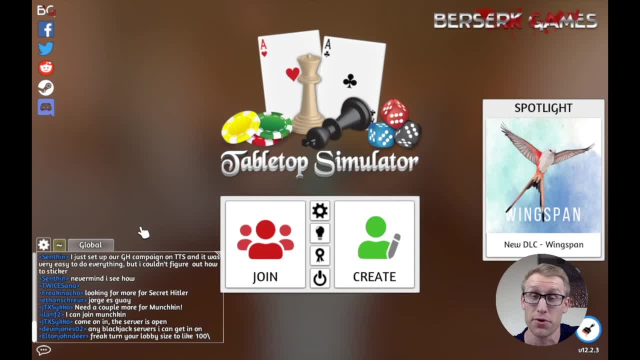 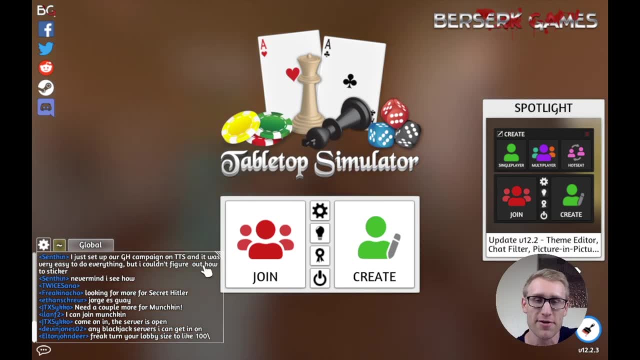 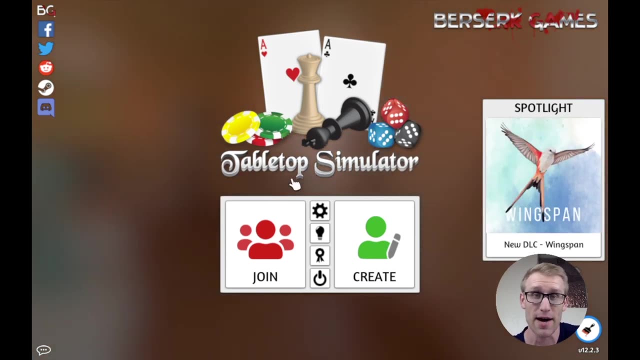 you might hear some white noise. that's actually my computer fan because my MacBook Pro gets working pretty hard when I run Tabletop Simulator. But Tabletop Simulator is a piece of software by Berserk Games that does exactly what the title says, which is simulates a tabletop. 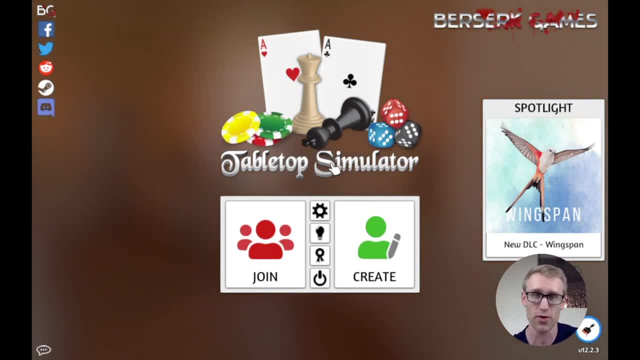 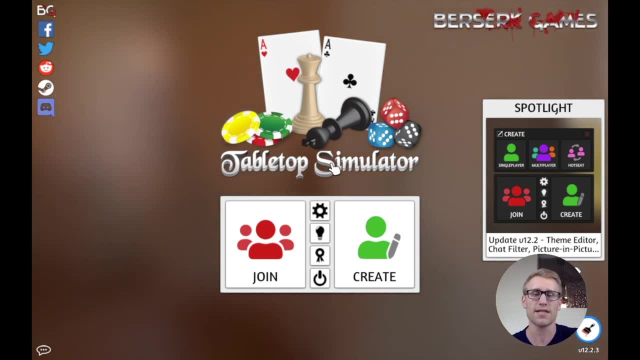 Now what that means is when you're playing a game in Tabletop Simulator- unlike, maybe, a video game- implementation of whether a video game or a board game- Tabletop Simulator isn't really enforcing rules, Just as if you were sitting at the table playing games with your friends. 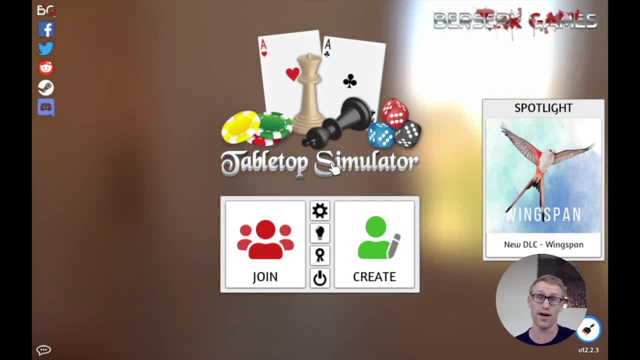 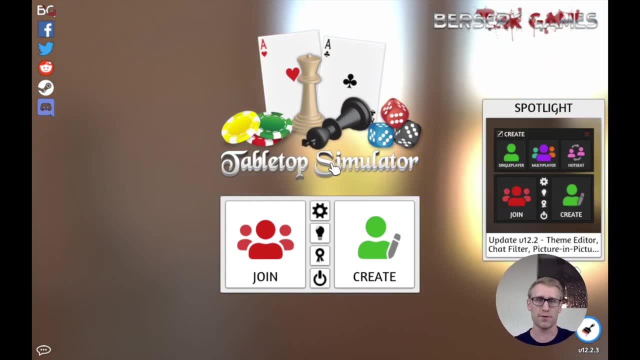 Tabletop Simulator will let you cheat. It'll let you do whatever you want. It'll let you flip the table, It'll let you throw things. It's simply like giving you a physical environment to play games in. And so why is that useful for us, you know, as game designers? 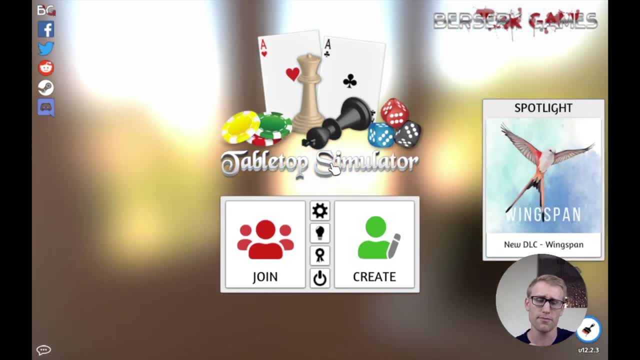 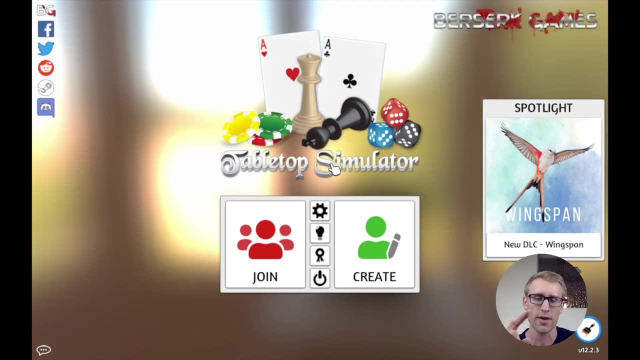 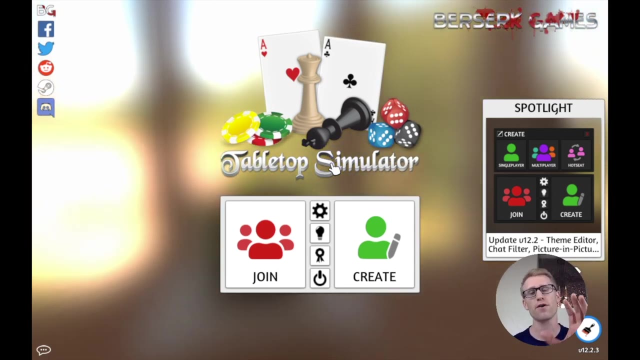 And I think there's two major reasons. So the first one is that if you're able to get your games prototypes into Tabletop Simulator, the first big benefit is just a resource benefit, both with time and money. So if you have your game in Tabletop Simulator, 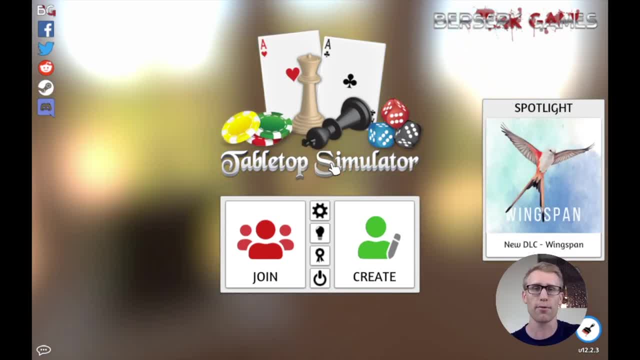 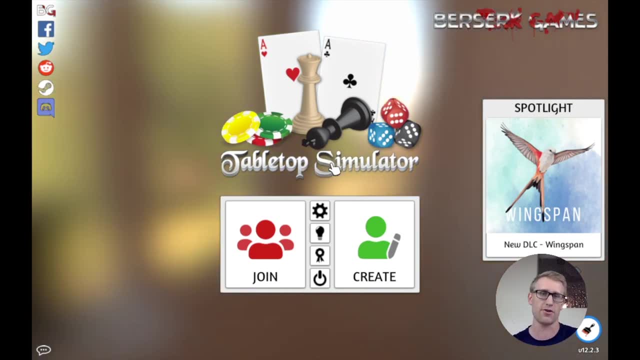 you can easily just start it up if you want to do a play test, and there's going to be zero setup. You're going to have your module saved and you just load it and the game's already set up When you're done playing. there's no teardown. 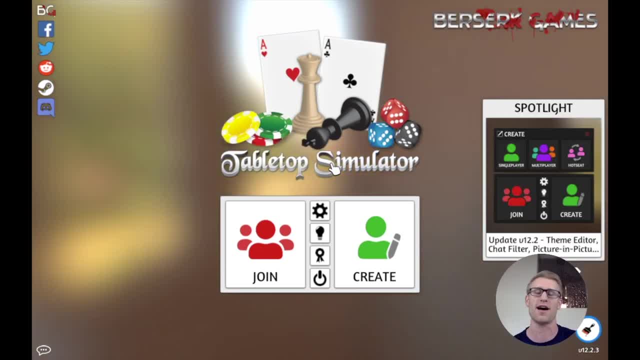 You just exit the game. So it helps that loop of just not needing to set things up on the table and get that all ready. Additionally, as you make iterations in your game and you make changes, you don't necessarily have to be printing out new components and gluing things and cutting things. 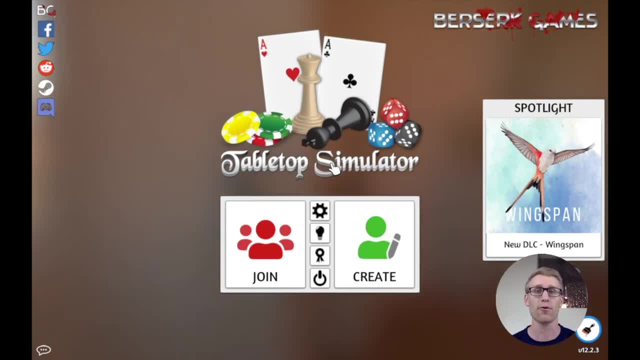 You can just import new assets into your module and be able to test the changes that way. So it really helps on that resource front. The other huge benefit is it allows you to play test remotely. So if I have my game in Tabletop Simulator. 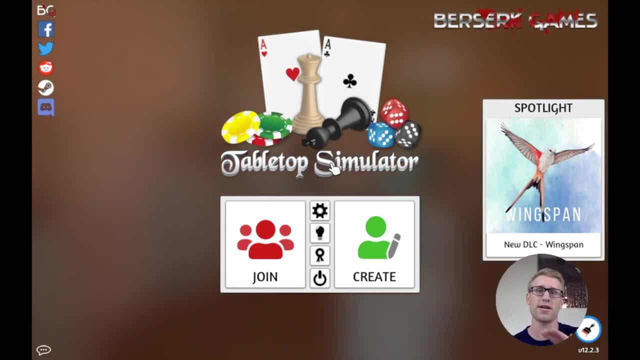 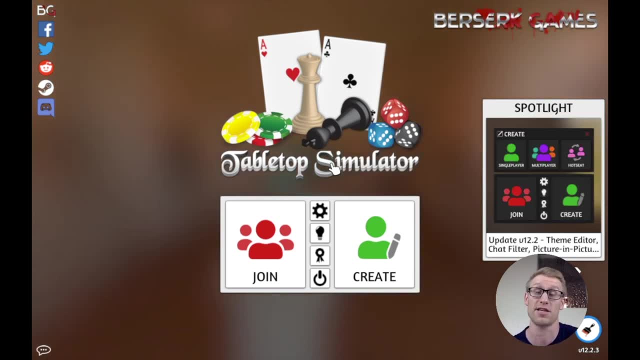 I can play test with somebody that lives in another part of the world by just simply getting them also onto Tabletop Simulator and we can voice chat and play the game that way, And that's a huge benefit when you think about if the barrier to play testing is getting a bunch of people in the room together. 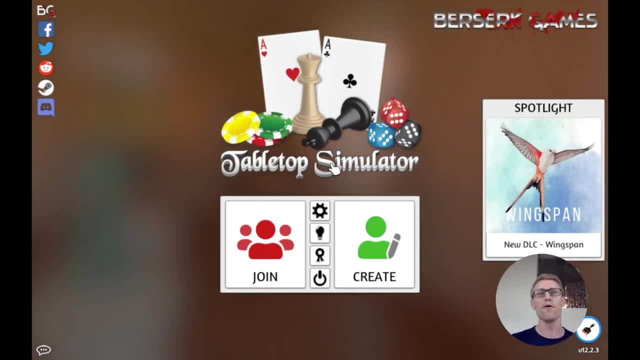 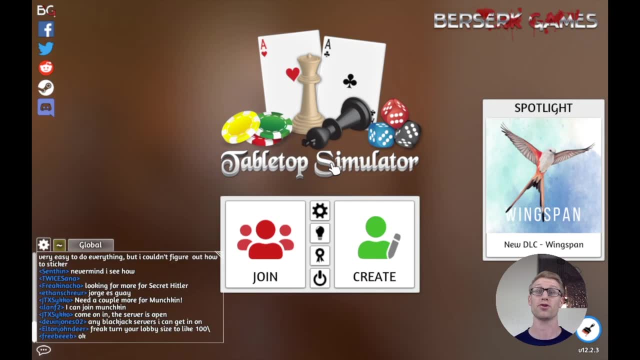 to be able to physically play a game. removing that barrier is going to just allow you to get more play tests in and play test with people that maybe you wouldn't otherwise be able to. So those are the two big, huge benefits for me. that kind of got me. 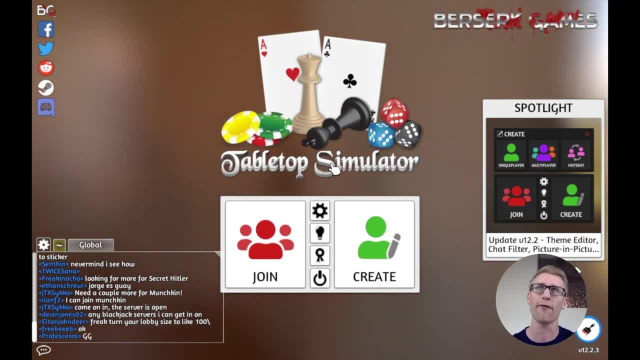 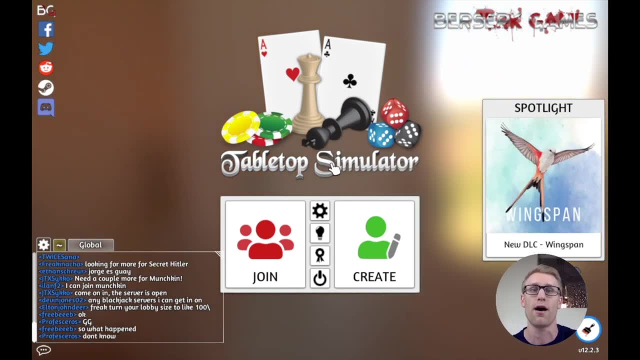 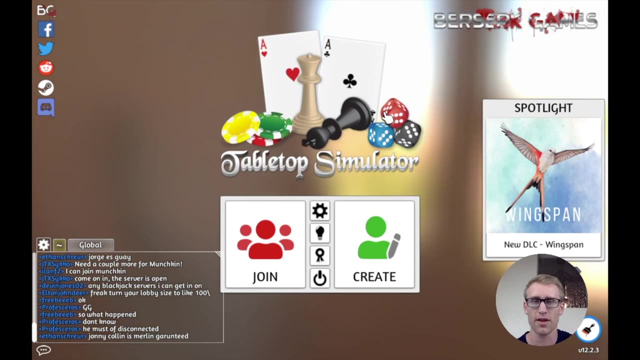 wanting to invest more in Tabletop Simulator, And I think they're compelling enough that any game designer could potentially benefit from learning how to use Tabletop Simulator for prototyping their games. So let's dive in here A little bit And there's kind of two skill sets you're going to have to learn. 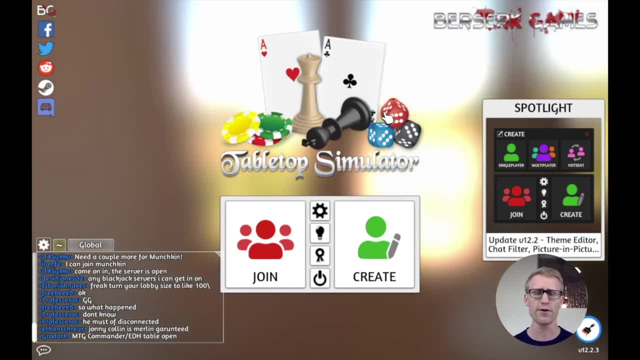 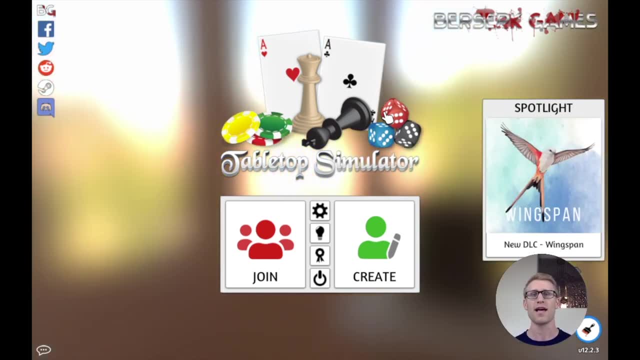 to be effective in prototyping in Tabletop Simulator. The first is just using Tabletop Simulator and the controls and moving around and interacting with the game itself, And I'm not going to really talk about that in this video. I'll link some resources below. 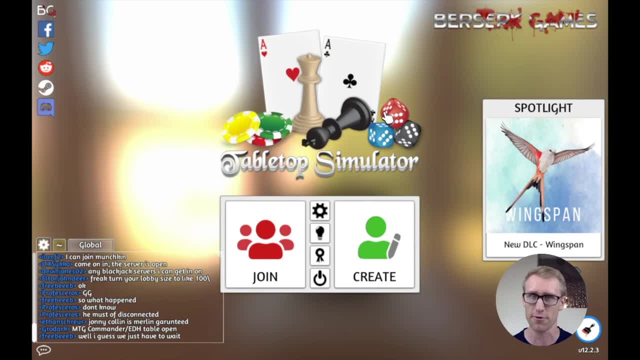 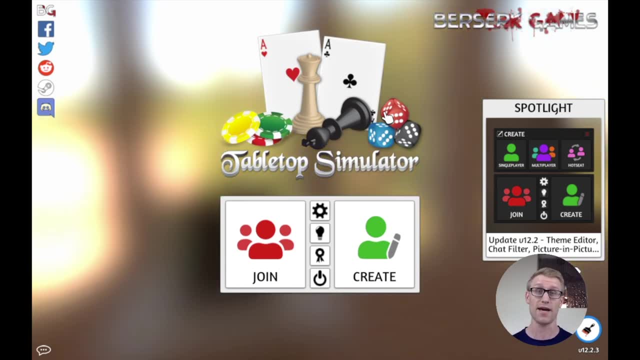 But that is something you should be aware of, that it's probably not going to come super intuitively right away. You're probably going to need to mess around a little bit and get comfortable with it. But it's worth learning those shortcuts And getting comfortable, because you're just 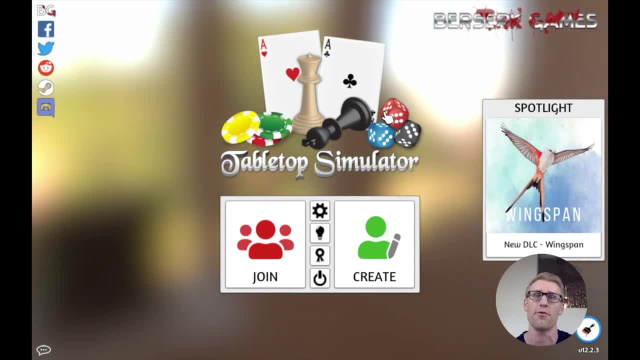 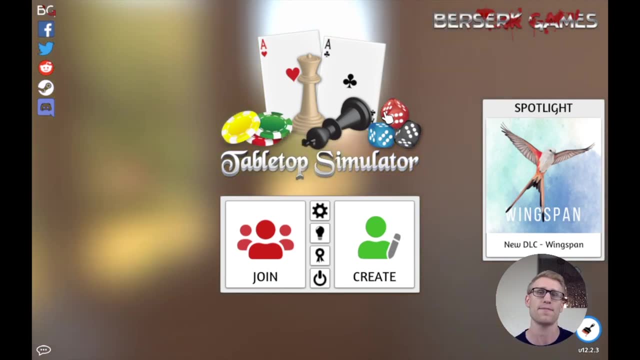 It's a quality of life thing, right As you use the software, you don't want to constantly be frustrated by it. But the second piece is just learning how to import games into Tabletop Simulator and prototype and do different things to make your prototypes more effective in Tabletop Simulator. 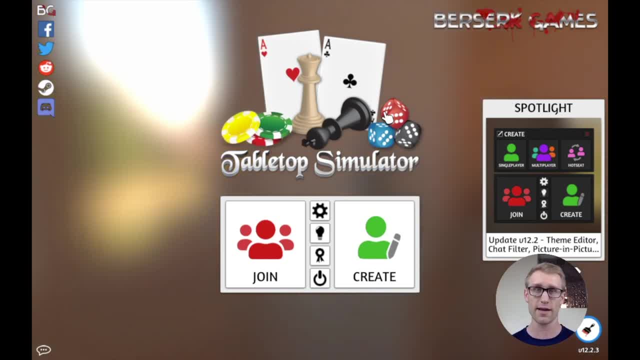 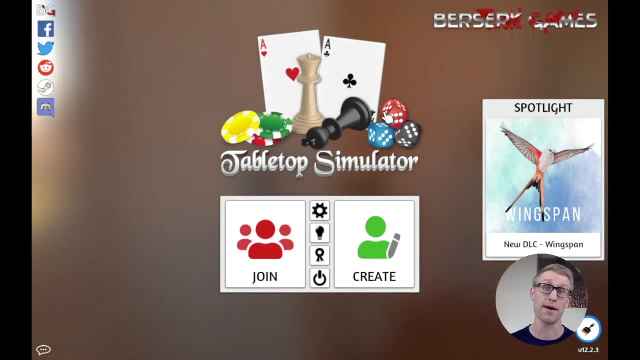 And so that's going to be more my focus in this video. I'm going to just go over some really, really basic stuff and just get the basic idea And then hopefully it can be a launching pad for some future videos where maybe I go over some more advanced topics. 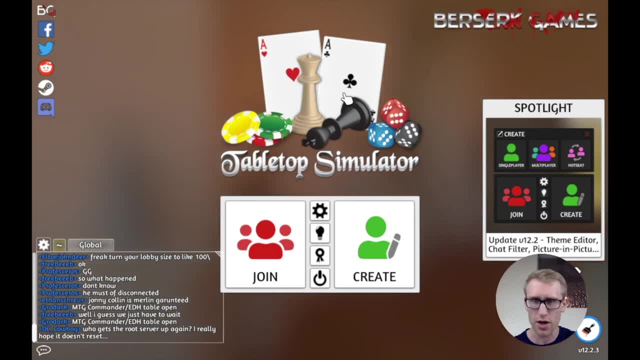 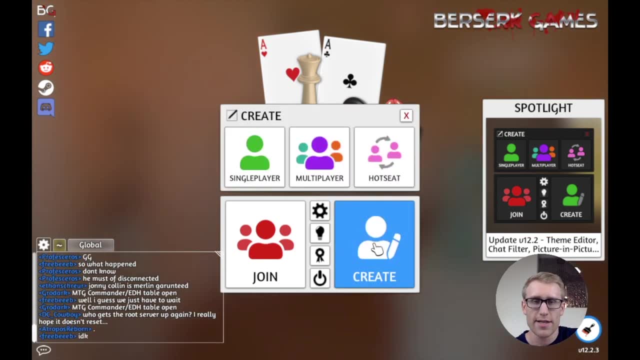 or kind of whatever people are wanting to see. So let's look, We got Tabletop Simulator open here. When you open this, you're going to want to create And it's going to give you a few options for single player multiplayer, hot seat. 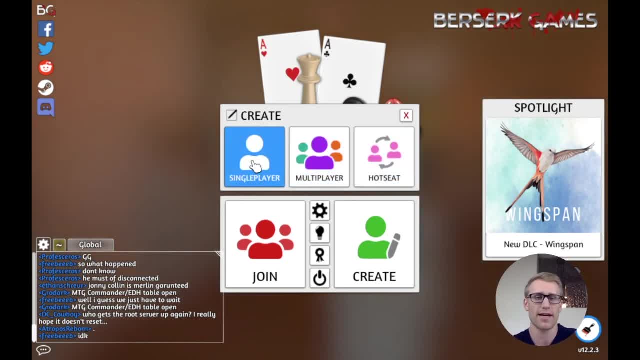 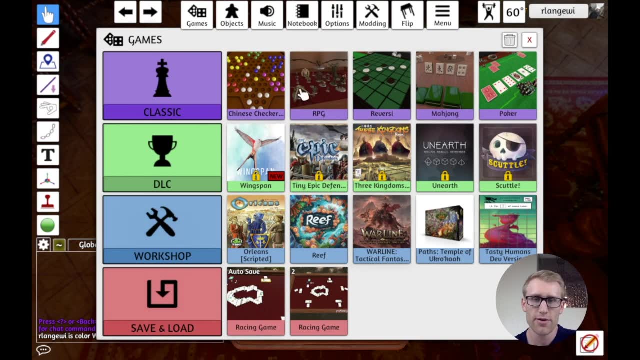 We're just going to do single player here. So this is like if I was going in and I wanted to make a new mod for a prototype. I'm working in. You're going to get greeted by this whole menu here, which is going to give you a bunch of different games that you're going to want to make. 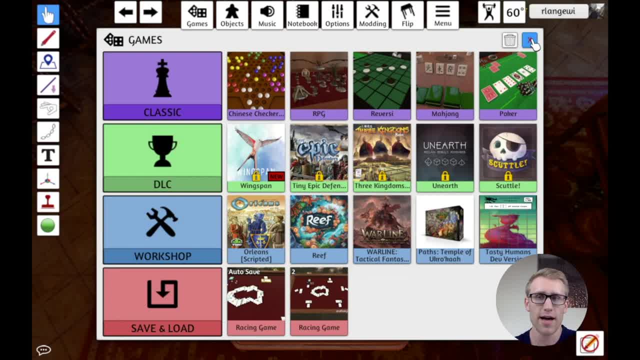 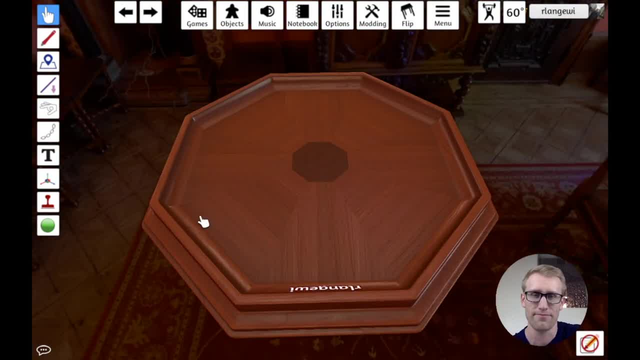 You could open. In this case, we're just going to X out of this, And so this is going to get us into kind of the Tabletop Simulator environments And I think it just throws you in with a random table and a random background. 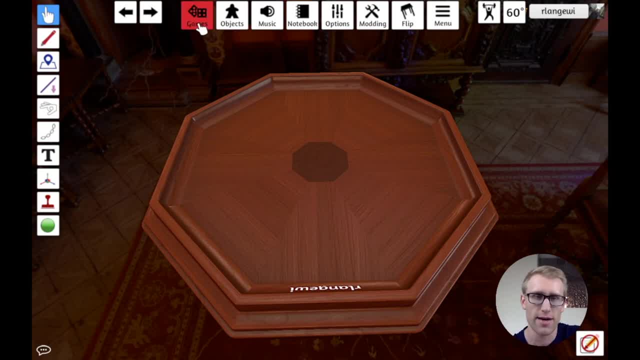 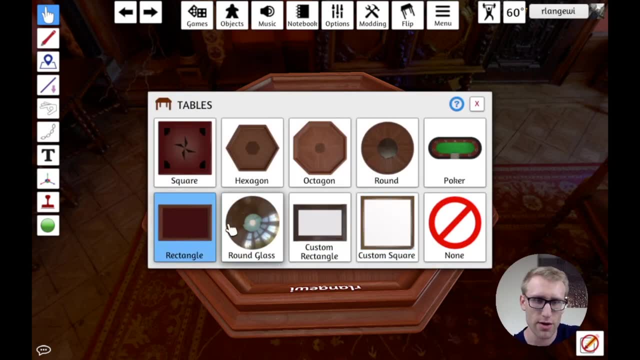 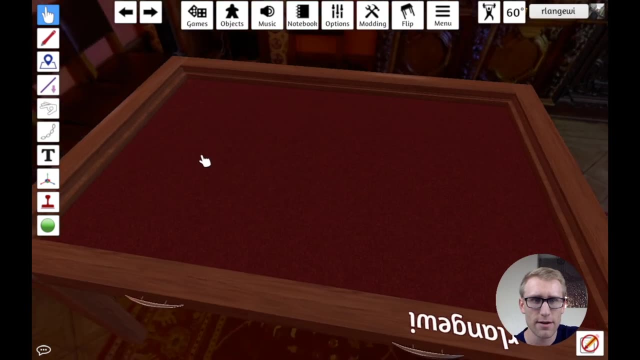 So I usually like using the rectangular table. So I believe if you go into objects and tables, you can pick whatever table you want. So I usually find myself using this one, And so I now have This table here that is basically a blank canvas for me to do whatever I want. 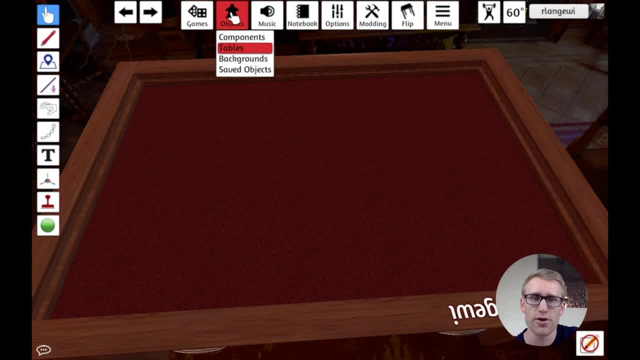 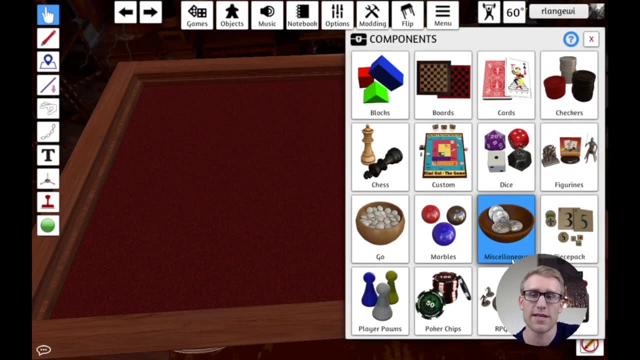 Now, if you go into objects here- and this is kind of a main menu you're going to be using to bring any different objects into your game- If I click components I'm going to be given a bunch of different options of things that I could put into my game. 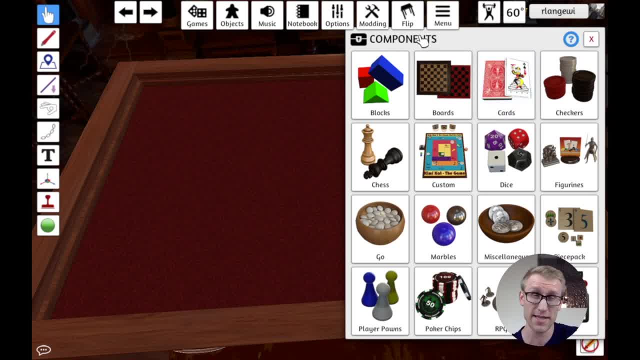 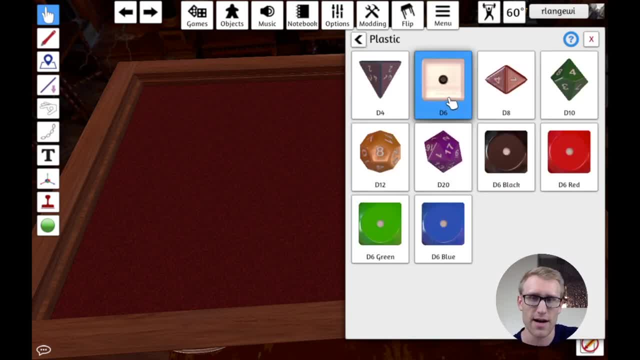 And so one of the things that you have available to you is just kind of basic game components that you might want. So a good example of that is dice. So like say I, you know, wanted some D6s. I can just put these in the game and you'll notice we have a nice die here now. 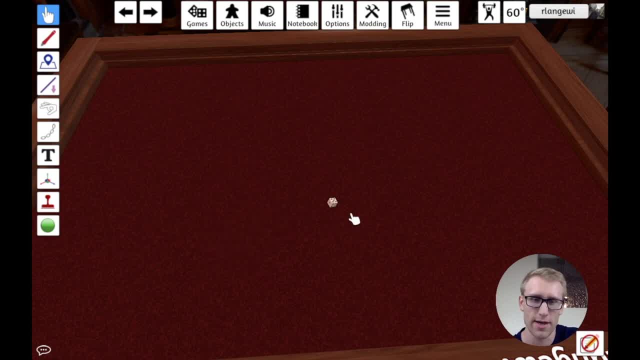 And I can. This is a physics environment so I can throw this around the table, I can roll it. It has some, you know, some different shortcuts to do some things. Additionally, I can take this and I can copy paste it. 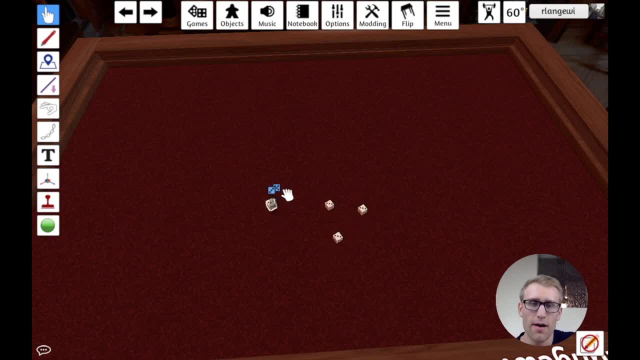 Copy paste it maybe. Yeah, there we go, And so I basically have infinite components here Right Which is kind of nice to be able to work with. So that's kind of. The first piece you have at your disposal is just all the built in components. 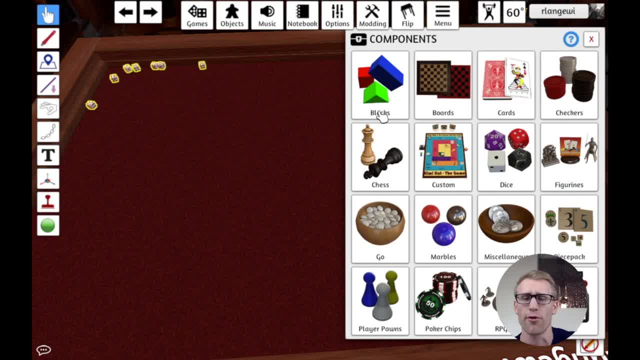 And so you can get some of the kind of basics like dice or other things, And there's some some other cool things that you can look into there. But the other big piece that you're going to want to look at is custom content. So this is any time you're wanting to import your game and do things that are custom. 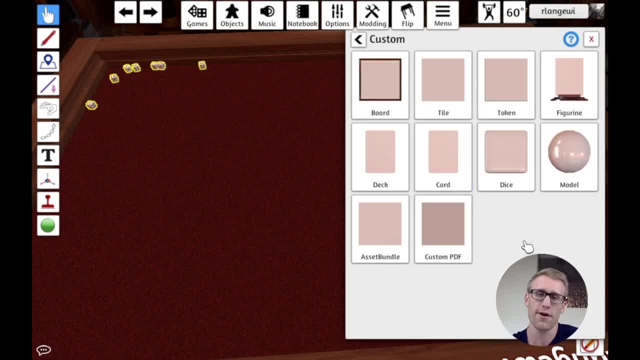 You're going to want to look in this menu. Now, this is going to give a few different options depending on, like, the kind of component that you're wanting to import into the game. So you'll notice, The first one is a board. 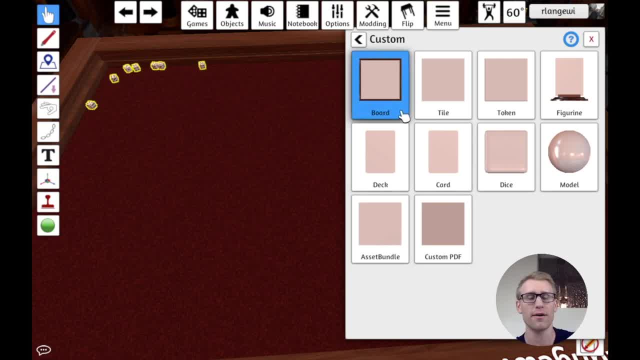 I actually don't find myself using this one very often. It'll basically import, you know, your game board with a big wooden border around the outside. I don't know, I'm not a huge fan of that aesthetic, So I typically just use the tile component for boards as well as other things that are. 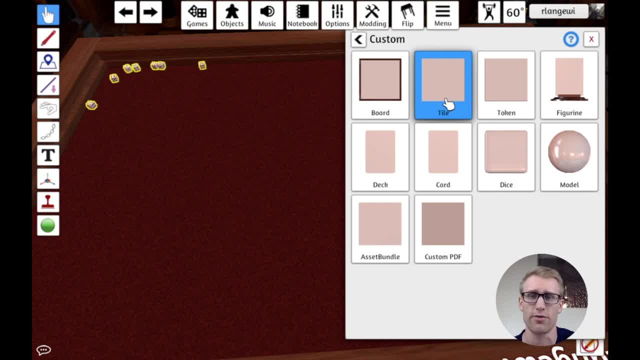 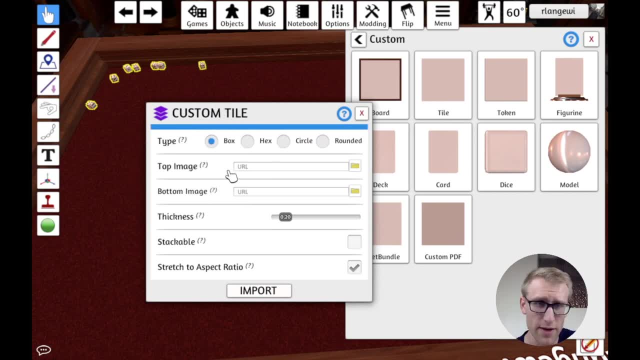 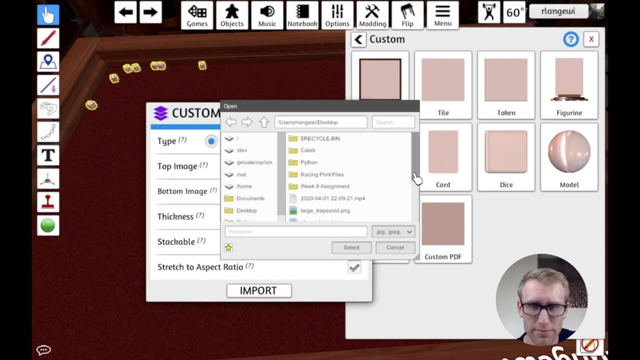 you know similar, So let's go ahead and do that. So if I click tile, this is going to give me a few options for a custom tile, And specifically, I want to import the image for my board, And so I'm just going to be using some examples here from a prototype that I've been working on. 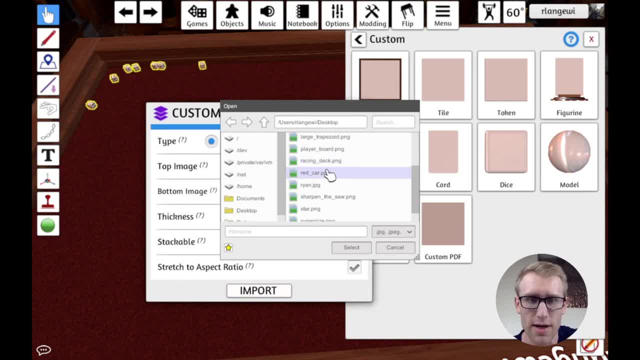 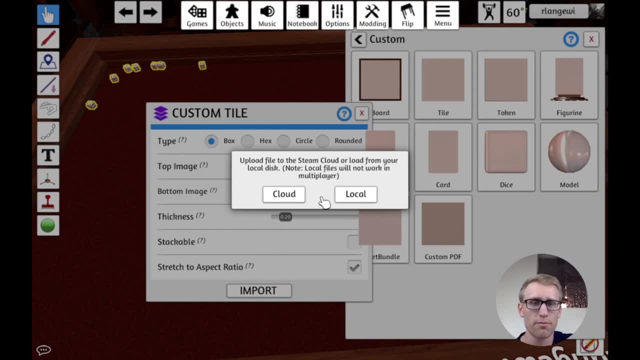 I think a lot of these assets are actually outdated, but they will do the job here. So let's get a player board and I'm going to select that And you'll notice that it asks you: do you want to put this image to the cloud or local? 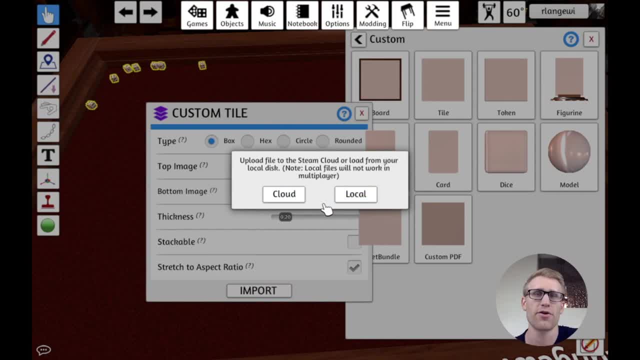 If you were just working on your mod locally and you know you're not planning on sharing it with anybody anytime soon, you could store locally. But by storing in the cloud you'll notice if I click upload here it's going to give. 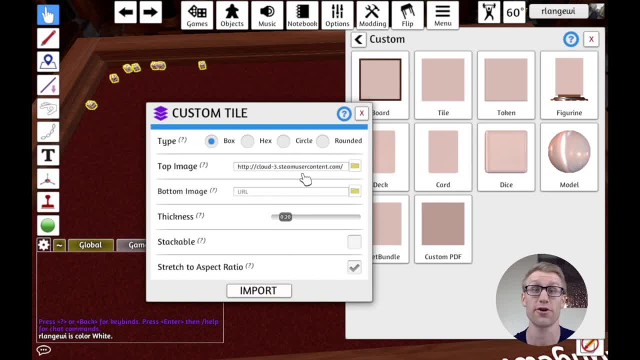 you this URL to basically where it's now hosting your image in the cloud with Steam, And so that way, if you later want to play the game with somebody else, they're able to pull down all those assets and have them appear where. that wouldn't work if it was. 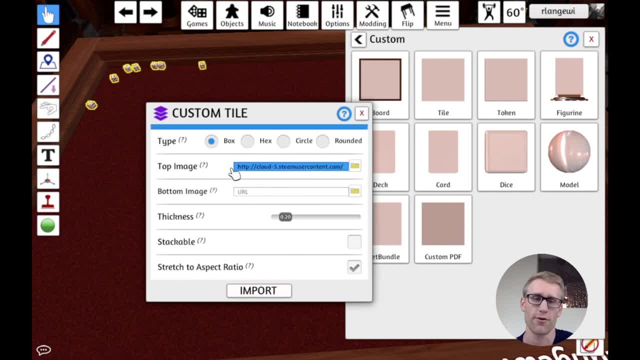 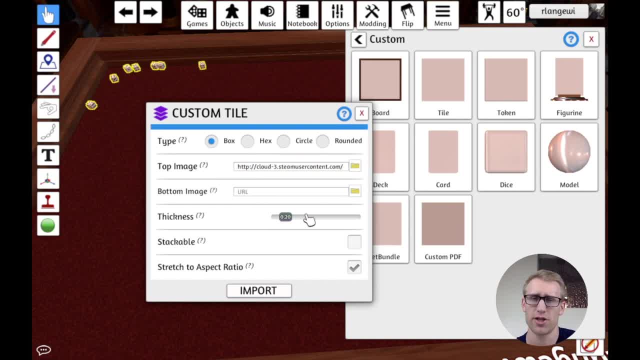 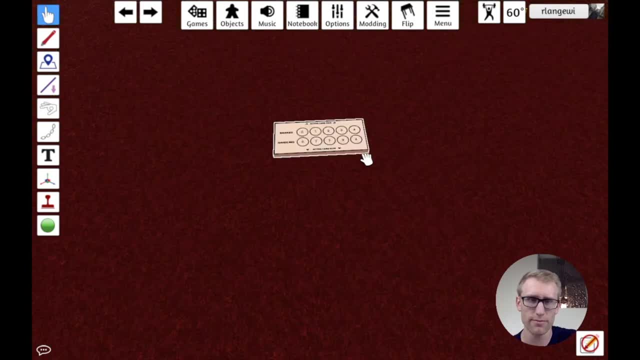 And then I'm going to be able to define the thickness, which is something I can also change later if I would like These other options look good. So let's just see what happens if I import this. So you'll notice, I have a new board here which simply has the graphic. that was just 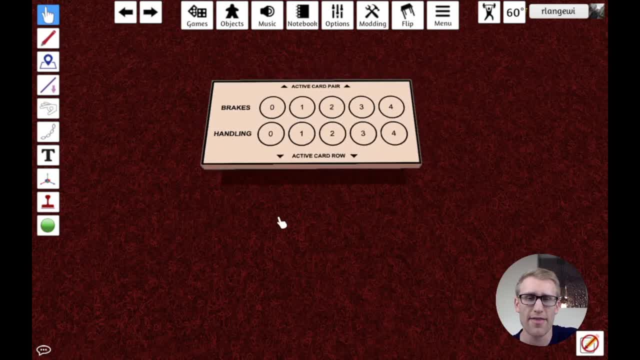 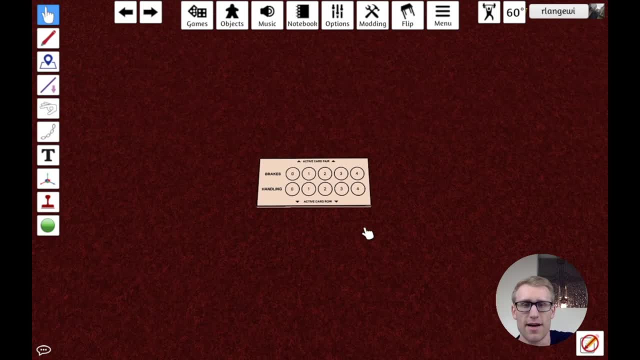 you know a JPEG or PNG image on my computer And this is now something that I can move around in the physical environment. I can flip it. it just use the same image for front and back, since I did not give it a back. I can also do. 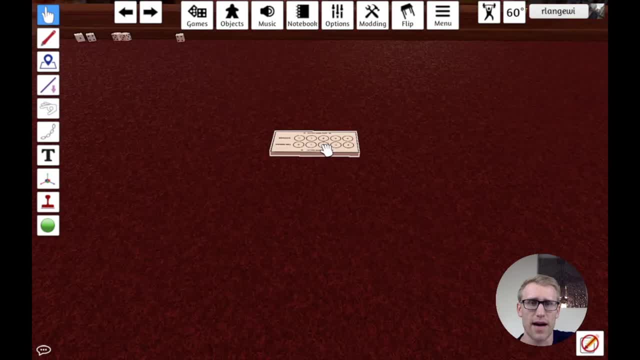 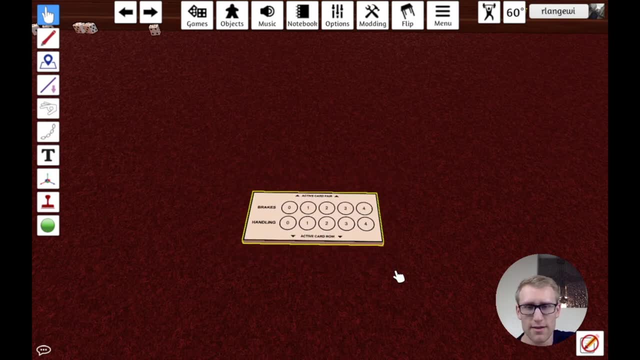 some things like changing the size. Maybe this isn't how big I want it. I can select it, and if I do plus on the keyboard it'll get bigger, And if I do minus it'll get smaller. I can also do that. 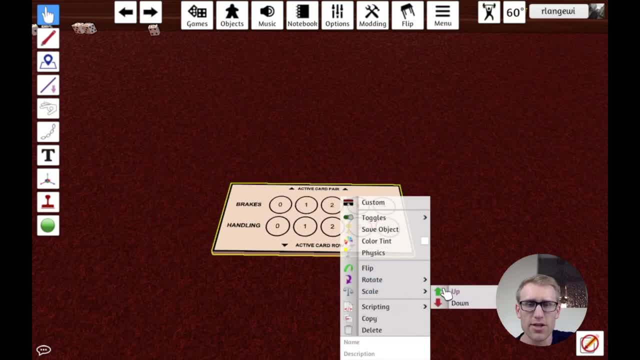 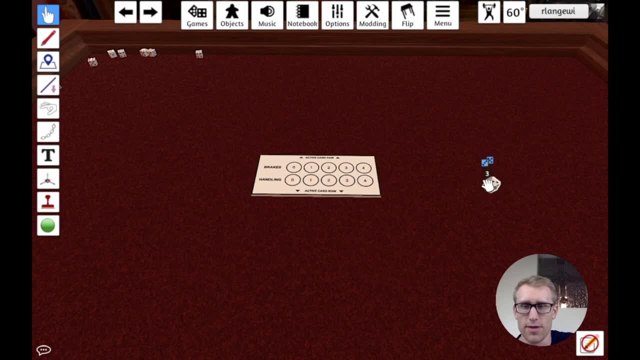 with the right click menu to scale it up and down, And so I can get everything to kind of the size I want to do. So maybe I get this to what I want, but maybe I need a few of these boards I could copy and paste this. Oops, my copy isn't wanting to work here. I can copy it and paste it. And now. 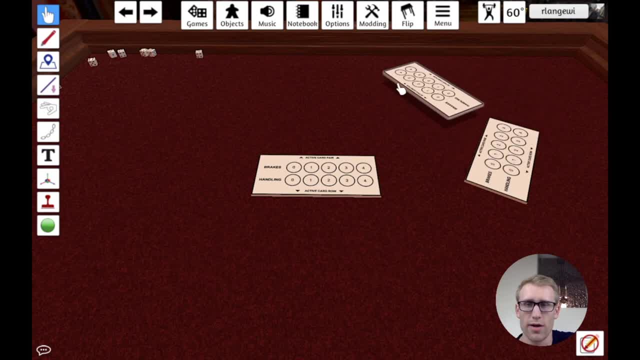 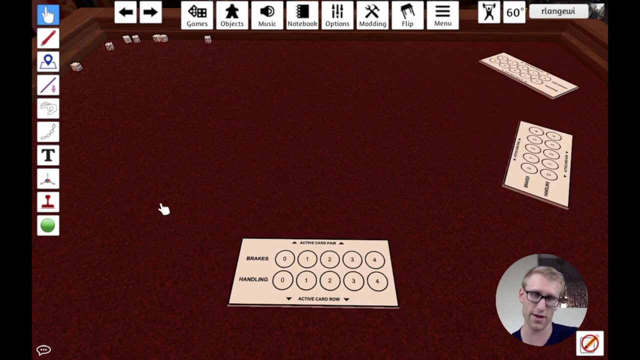 I have this available, like if other players wanted to be using it. So that's a basic example of just quickly getting a board into the game And, as if this was a game board, I could make it as big as I want to make it. 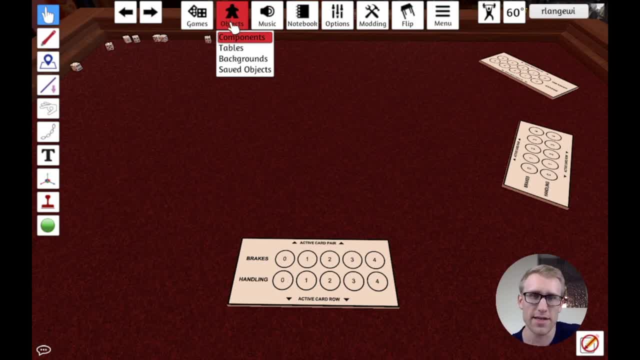 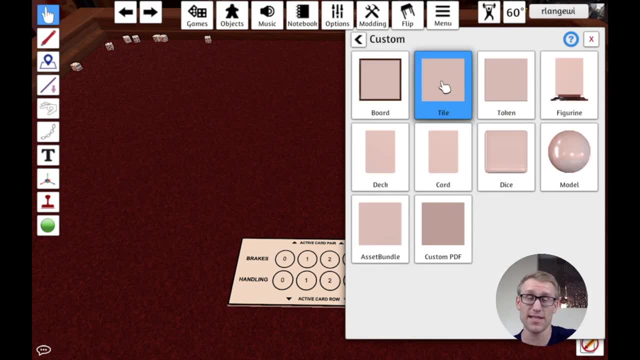 So suppose we wanted to just import, like a player piece or something. Similarly, I find myself using the tile option a lot Anytime. it's kind of just a piece that's flat, whether it's a board or something smaller. tile is usually kind of my first go-to. I'll talk here in a moment about when I might use. 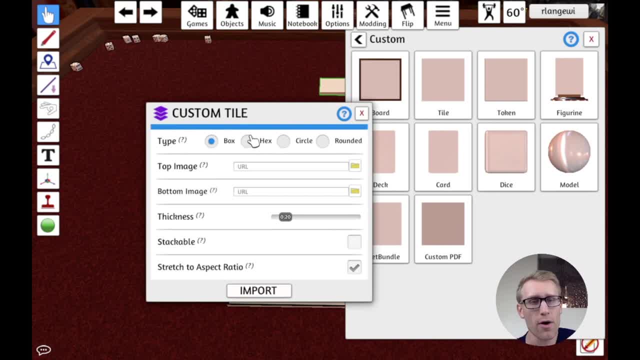 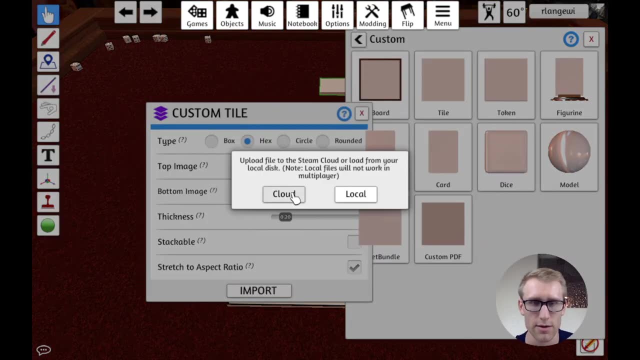 token. but let's go tile here again And maybe I want this to actually be on a hex, so a hexagonal piece instead of the square. So here I'm going to pick again, and let's pick my red car here, Store in the cloud And we'll leave. 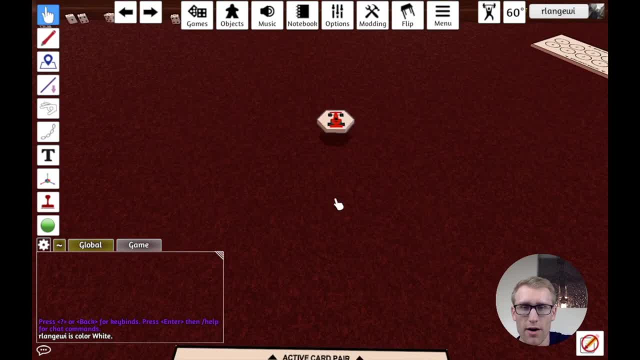 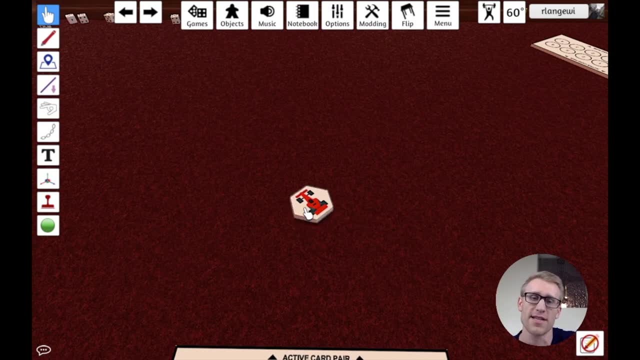 these options the same and import it, And you'll notice now I have my car. that was just in the original graphic, for this image wasn't a hex, right, It was just a square image, But because I selected hex, I'm able to get a piece that looks like this, which actually, for this particular 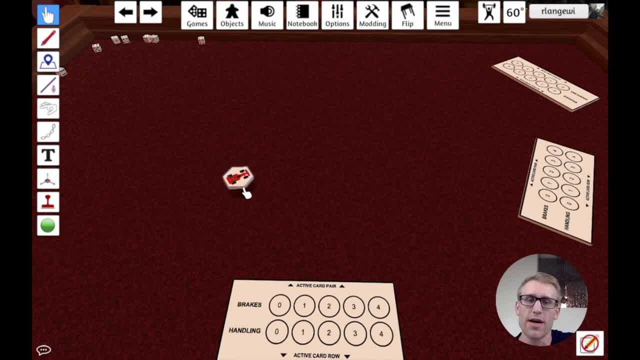 prototype is what my pieces ended up looking like, So I'm going to go ahead and make that a square, So you have some different options. You'll notice here when I'm rotating the pieces. right now it's rotating on a 60 degree interval. 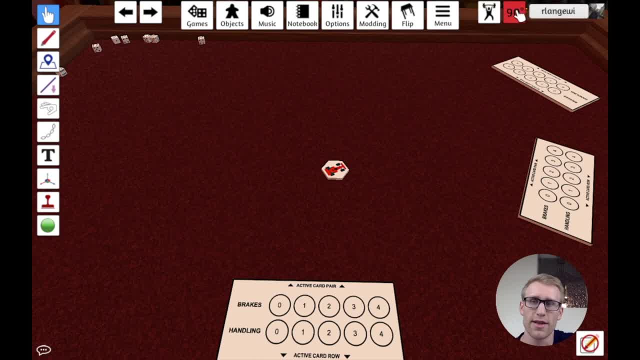 That's simply this option up here. So if I wanted that to be 90 degrees, I could switch that and it would rotate on 90.. Again, all this controls the controls of how to rotate things and flip things, and all that. 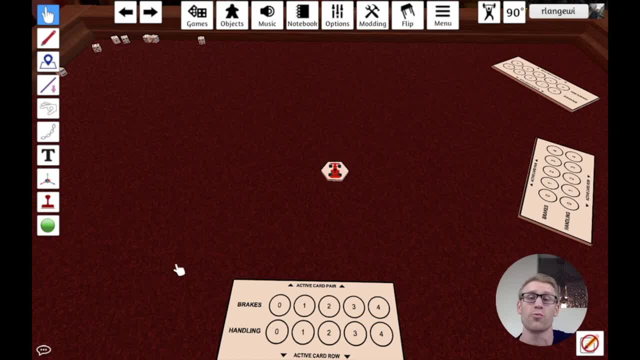 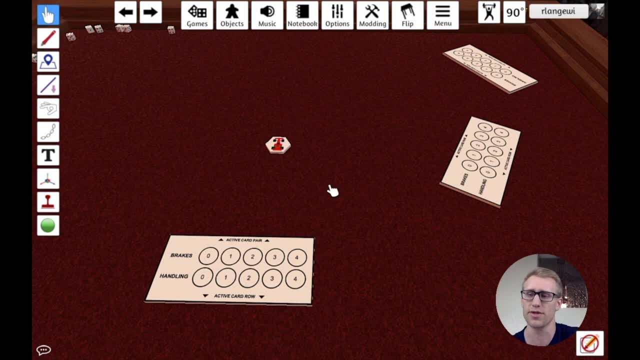 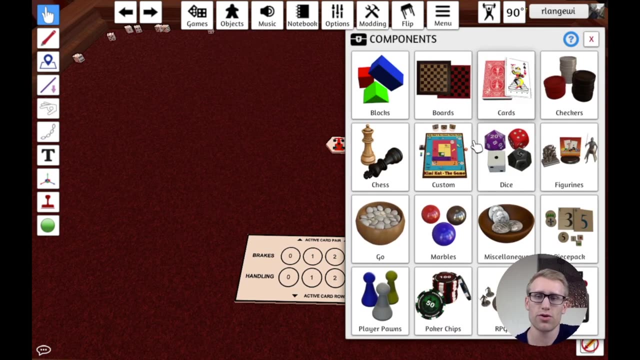 that's going to be something you're just going to have to get used to and learn. It's worth learning the shortcuts, And it really does start to become intuitive once you start just using it more often. So I mentioned that you may want to use a token, So a token is very similar to a tile. 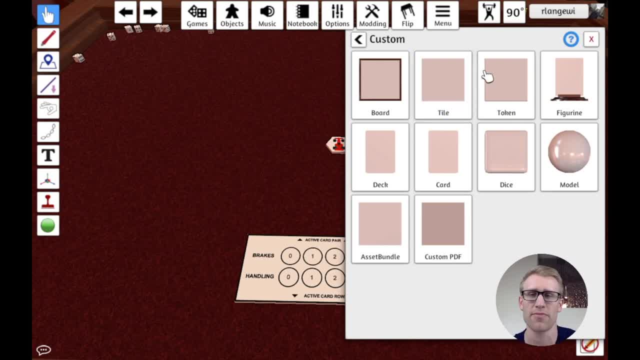 And if you look in Tabletop Simulator's documentation, basically, at least from my understanding, the big difference with the token is a token allows you to have kind of irregularly shaped tokens. Tiles are tokens, So if you have something that isn't a hexagon or a square, 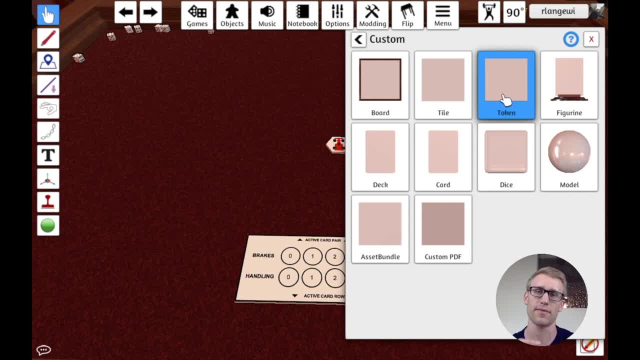 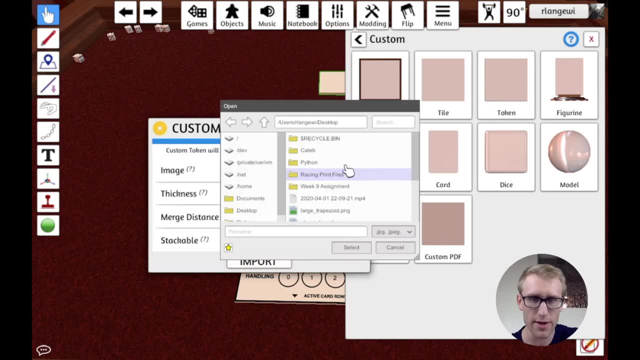 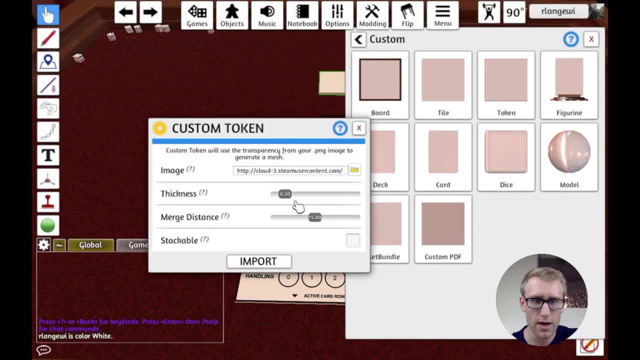 you could actually get that with a token and give it as a PNG. that has a transparency. So let's actually give an example of that. So if I did token and pick an image and I actually think this one should work, We'll upload that Thickness, fine. 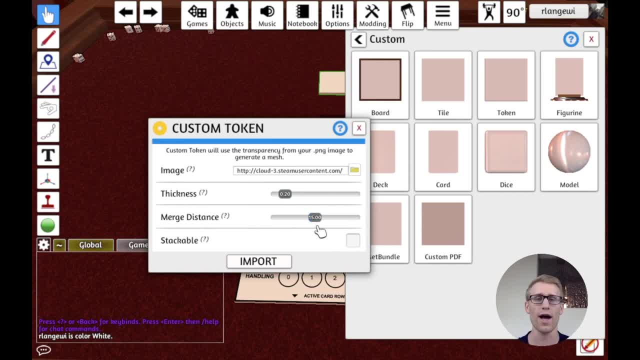 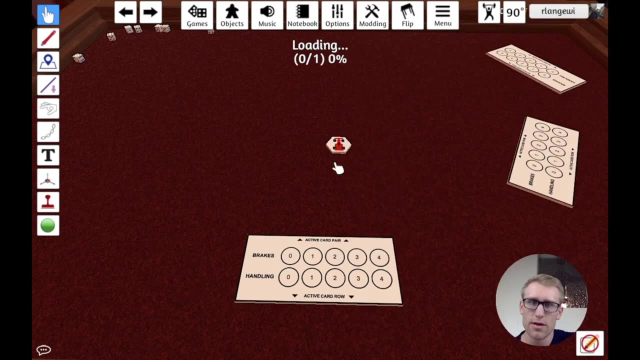 Merge distance. all this is saying is basically: with what accuracy do you want it to be? You want it to cut out? based on that transparency, If I want it to be really accurate, I would bring this down lower. I'm not too concerned about it, So let's just import that. 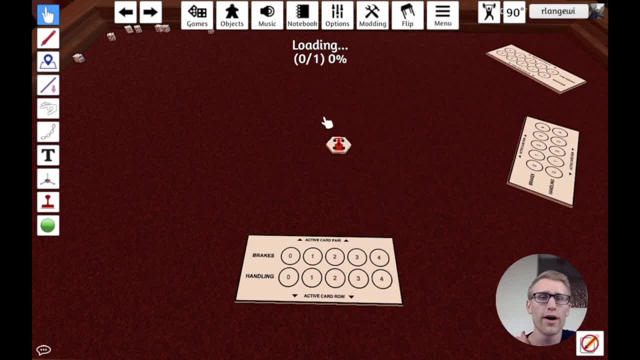 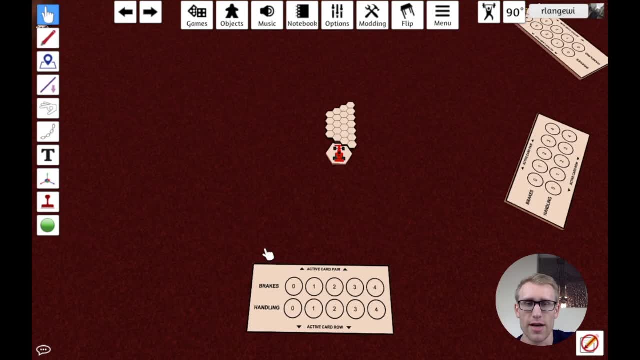 So we wait a little bit. It's got to think. So it's a little more taxing on Tabletop Simulator because it's got to actually cut out the transparency to figure out what this token looks like. But there we go, We got our tile here. 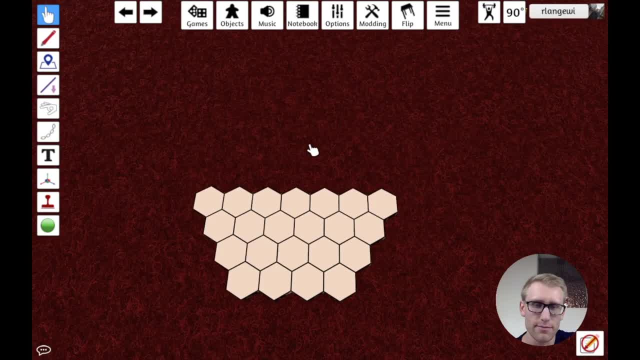 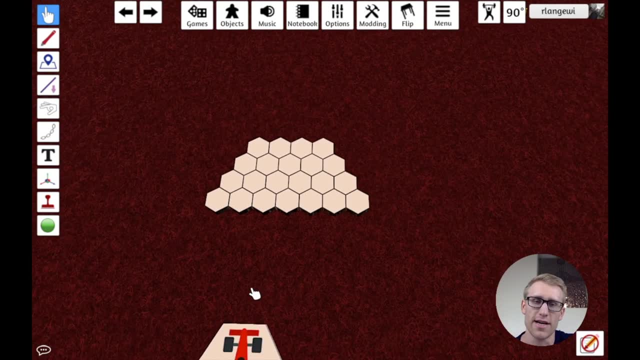 And so you'll notice, this is basically a tile piece that's made up of a bunch of hexagons, and it actually cut it out appropriately around all these hexagons. So if you have a piece that's like that, that needs to be like a very different shape. 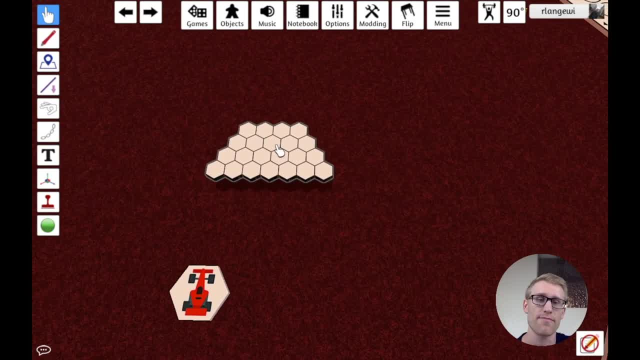 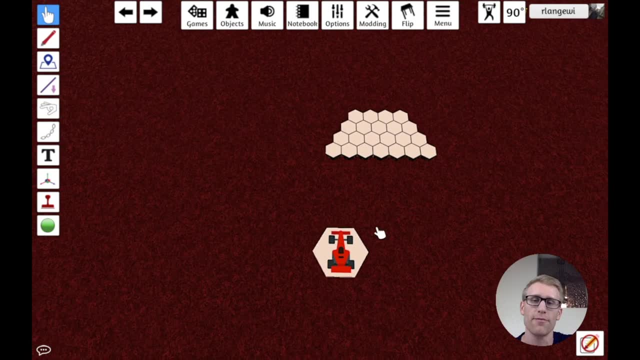 then token may be your way to get that into the game. However, there's no options for tokens to be double-sided or to have different graphics for both sides. You would need to use a tile. So my recommendation would be: use tiles whenever possible, unless you want a regular token. 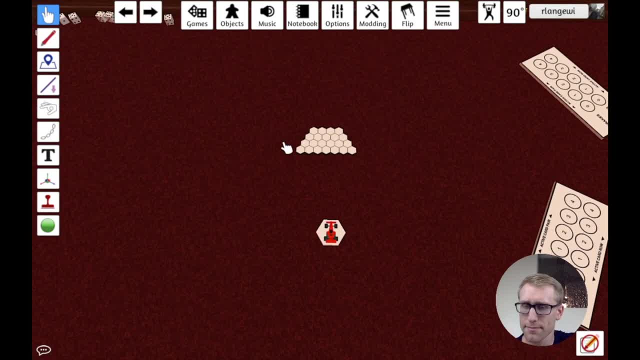 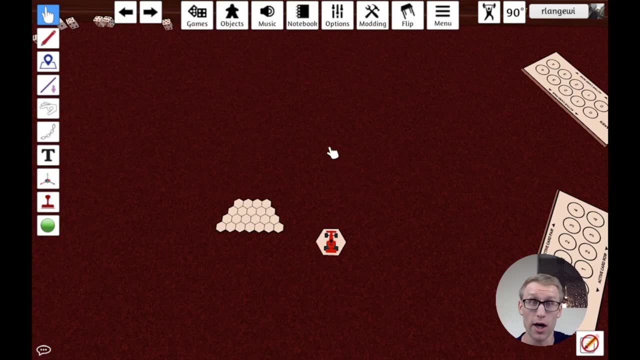 So you want to have a lot of different shapes and then use a token. The other main component or basic thing that you might want to import that I'm going to talk about here quick is cards. So a lot of games have cards And suppose we wanted to import a deck of cards. 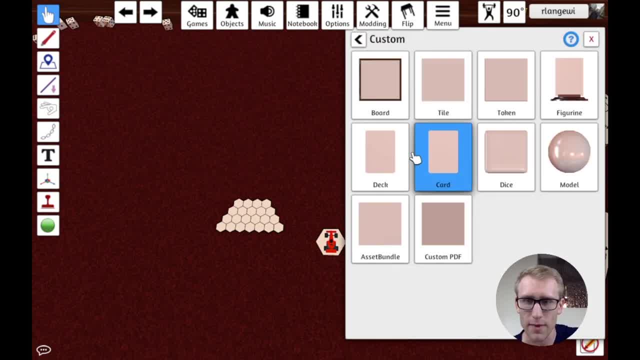 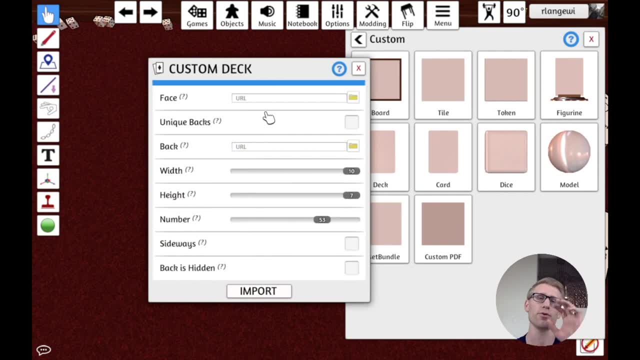 So if I go into components here and I go to custom again, I could import single cards, but I'm going to actually import a deck. Now when I import a deck, basically, Tabletop Simulator has a specific format that it's looking for. 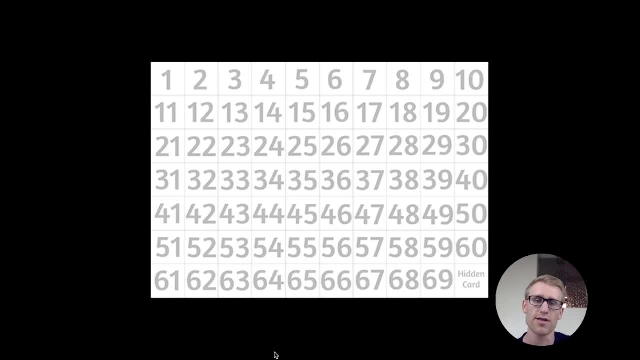 And I actually think I have it open here, so let's look at this screen. So this template is what Tabletop Simulator is saying. this is how you need to organize your cards for it to import it as a deck. So it's basically a 10x7 grid of cards, with the bottom right one being kind of just an empty card. 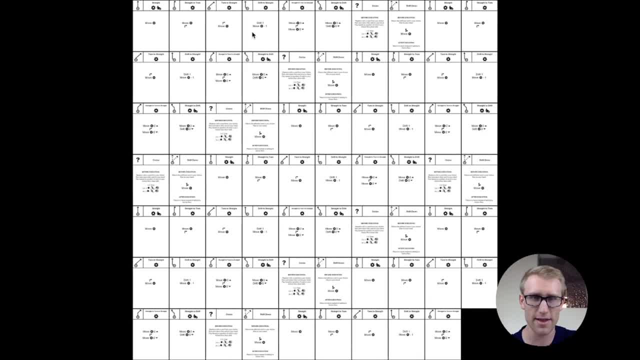 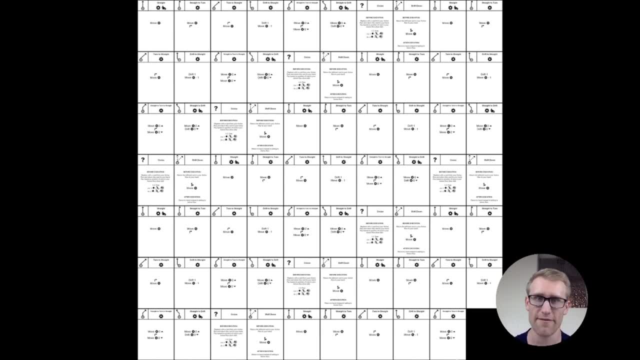 And so, as an example, I have this here, which is a bunch of cards that I have for this game, arranged in that 10x7 grid that it'll be expecting, And the actual ratio isn't as important as the fact that it's expecting. 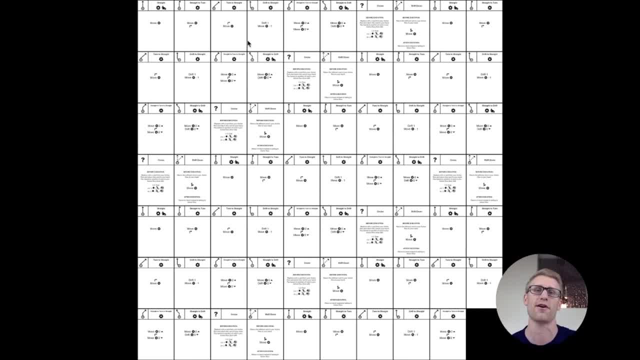 it's going to divide the width of your image by 10 to get the width of the card, and then the height by 7 to get the height of the card. In this particular instance, these cards are actually just repeated a bunch. It's like the same eight cards over and over. 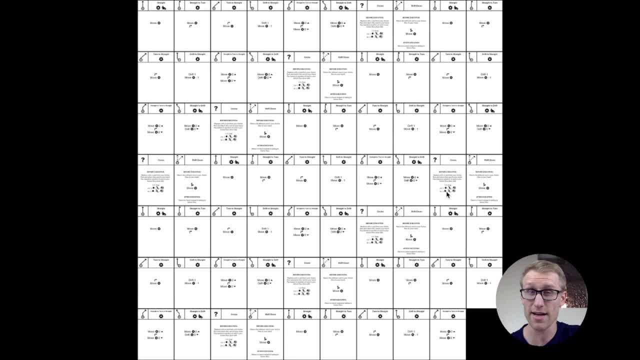 And I actually generated this using a program called NANDEC, which I'm not going to get into here, but I would love to, in the future, talk a little bit about how I use that tool, kind of in conjunction with Tabletop Simulator. But all you really need to know here is: this is an image. 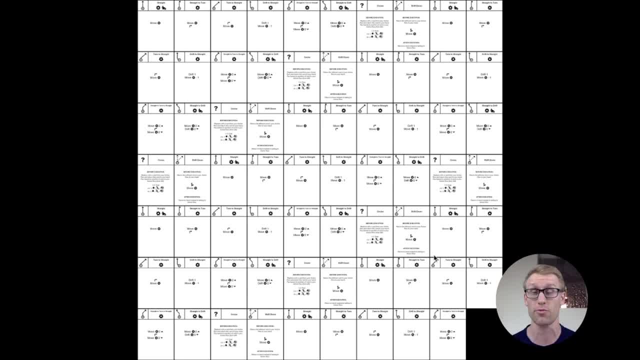 It's a really big image, And if you had a deck of cards that you want to import, you would simply need to align your cards into an image like this before you import it, using whatever Photoshop or GIMP or whatever software you want to use for that. 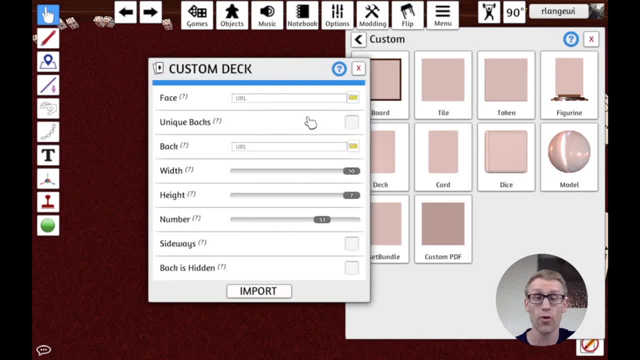 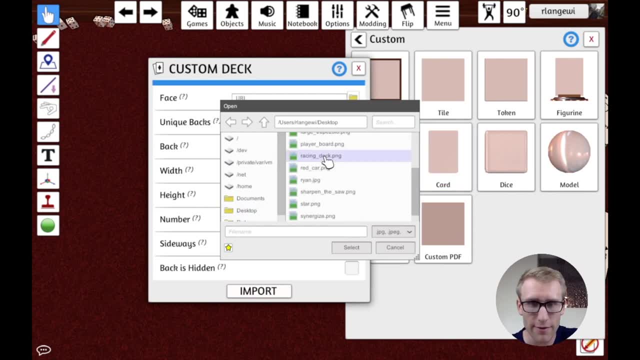 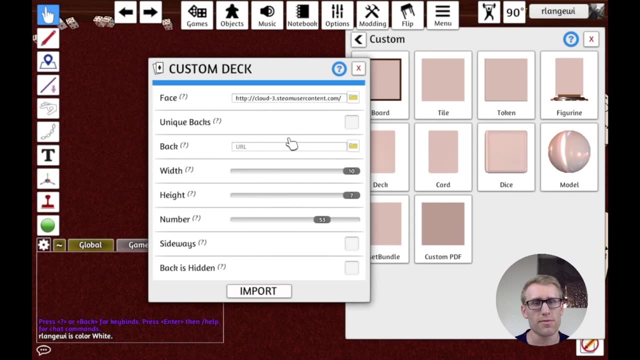 So once I have that, I'm going to in my custom deck here, going to select that image as my face. So if we look here, I have racing deck. I believe We'll do cloud again Upload. There's some different options here. 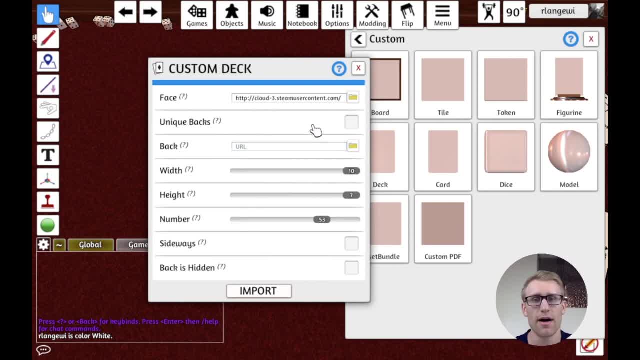 For example, unique backs would let me like if every card had different backs, then I would have to provide another similar image that has 70 cards where they correspond to each back. In this case I won't, And actually I don't really have a back of a card prepared here. 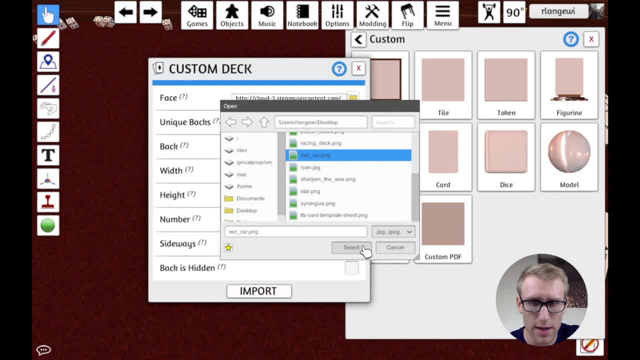 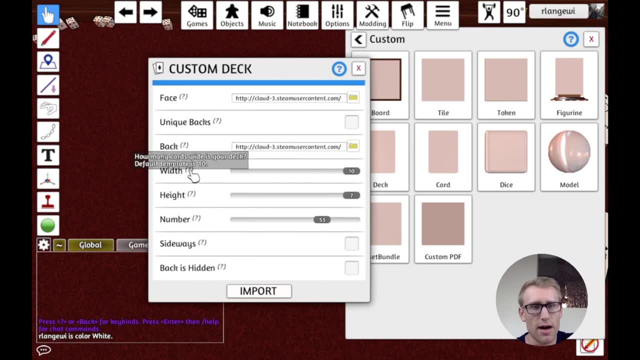 but let's just use the red card, Why not? So we'll select that, And so then this has got width and height, And so, yeah, I guess this is. you could adjust the template from 10 by 7.. 10 by 7 is the default. 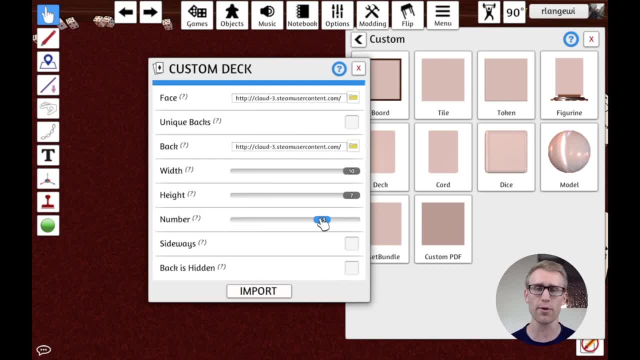 And then this is the number of cards. So, even though my template had, you know, the full 69 cards, in this case I'm only interested in importing the first eight of them, because it's just the same eight imported over and over. 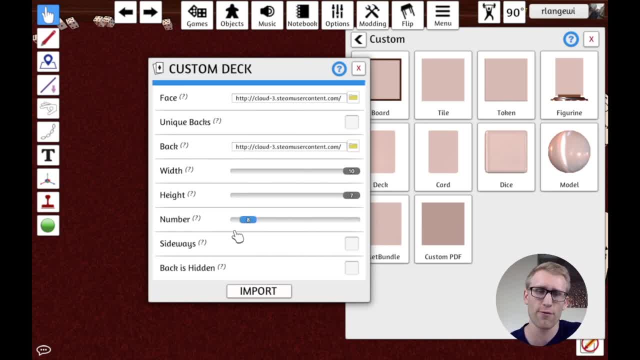 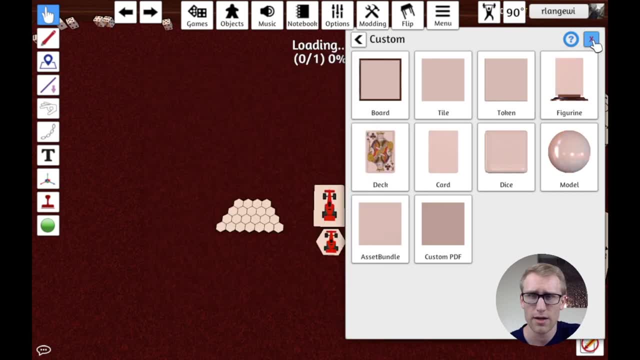 So you can. if you know how many specific cards you're looking for, you can adjust that here. Not concerned with these settings, So let's just go ahead and import. So again we'll see Tabletop Simulator working to load it into the module. 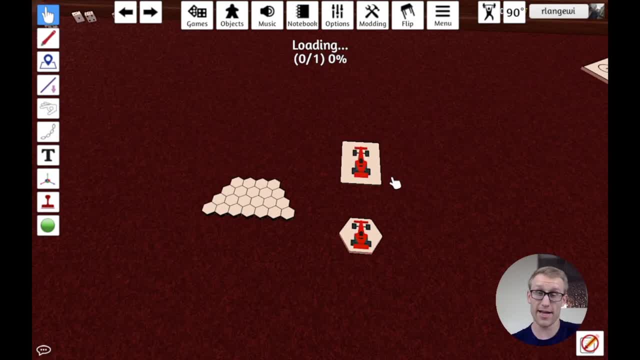 It's worth mentioning that once the cards are in Tabletop Simulator, they're just an object like anything else, And I can duplicate cards. I could copy the whole deck, And so what that means is, if your deck distribution has duplicates of a lot of cards, 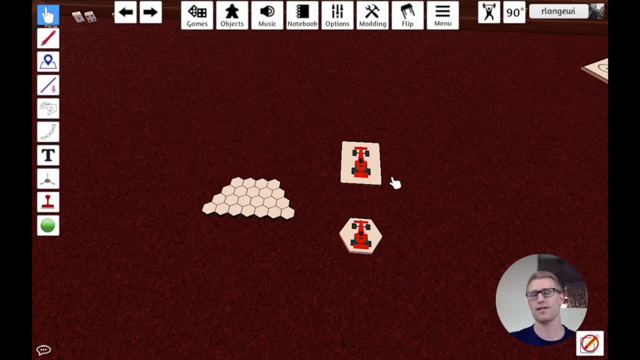 so a lot of games you know have a deck distribution. but there's, you know- take like Dominion, for example- you have a bunch of like copper coins and there's like tons of copies of that card. You would only have to import one copy of that card if you wanted to. 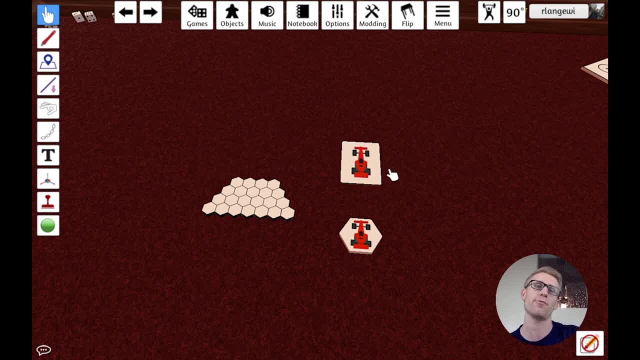 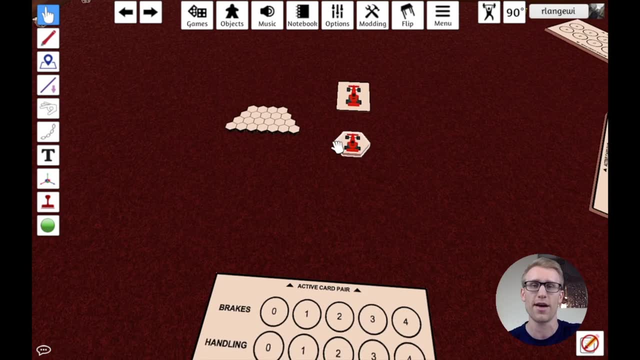 And then you could do all the duplication in Tabletop Simulator rather than doing all the duplication in your image file and having like tons of the same one clogging up your kind of 70 slots If you wanted to have more than the 69 cards. 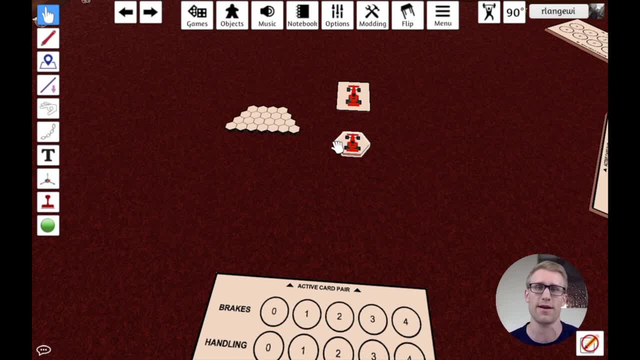 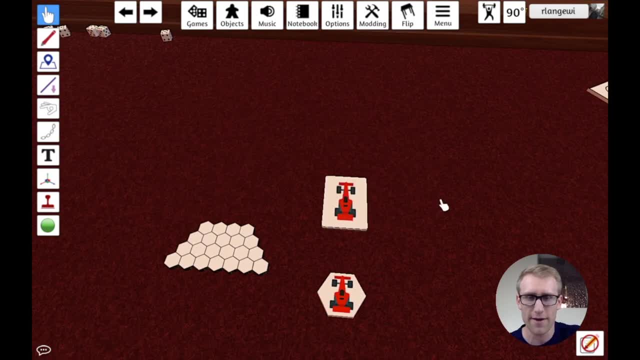 you would just have to have separate files and import more than one. Let's take a look at what we got here. So if I hover over here, it says that there's eight cards here, And if I draw one off and flip it, 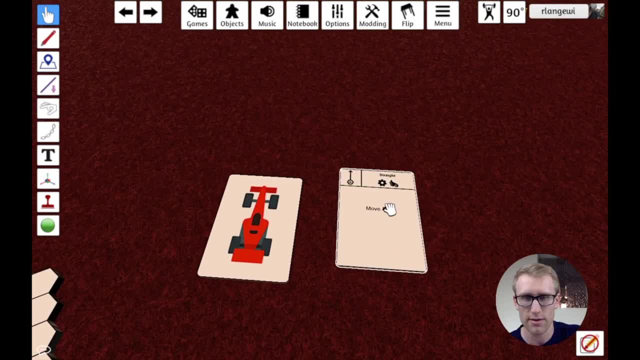 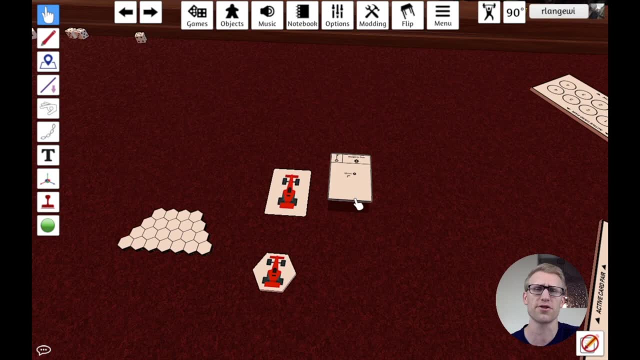 I can see that this is one of my cards that I had, And so I basically have a deck of cards here that can be manipulated and get all of the kind of features that Tabletop Simulator has for cards. So, for example, it supports players having hands that are hidden from each other with cards. 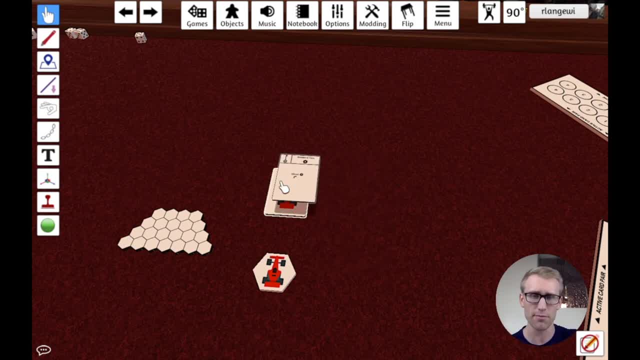 and playing cards, And I can put these all on a deck and I can shuffle the deck. So there's a lot of just basic features there. There's basic features that you would expect to be able to do. that I'm now able to do with these cards. 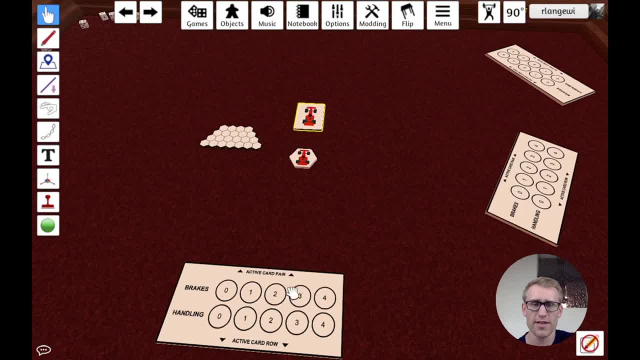 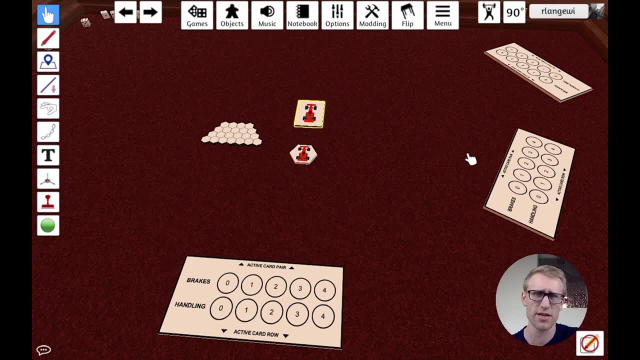 So that's kind of just some basics of you know. you can see it was pretty simple. Once you learn those, like you know two, three options, you can get most of the types of components that you would want into the game. 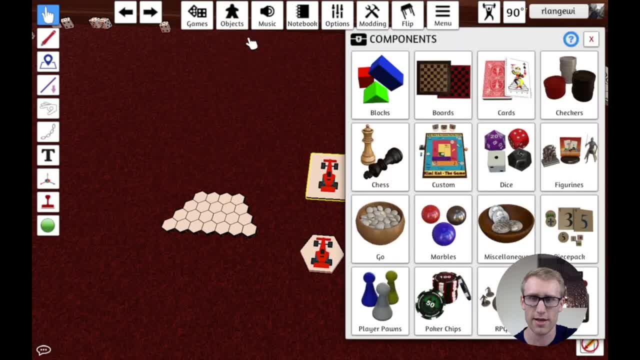 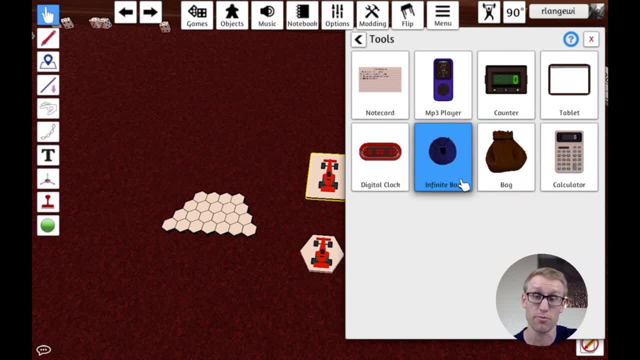 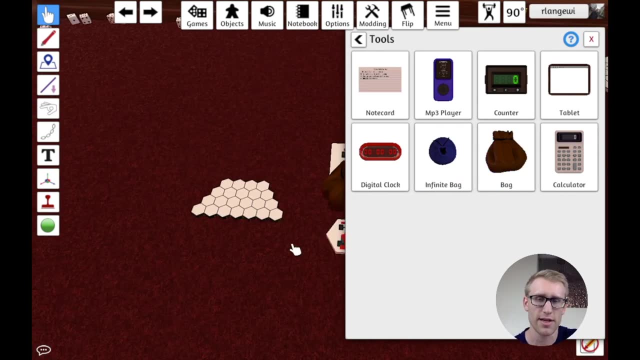 Another just good thing to mention, I think, is if we look here at Tools, a common thing I find myself using is the infinite bag. So if we brought a bag in, basically what that would allow me to do is like put tokens in it. 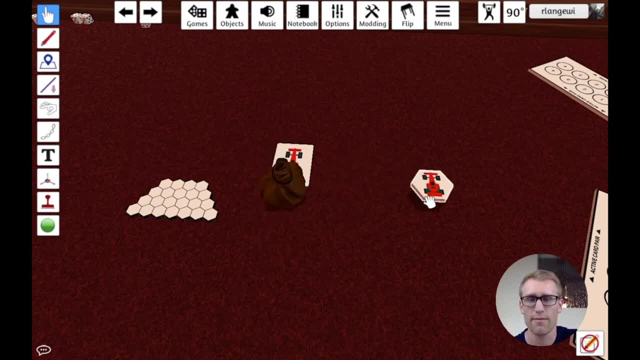 So I could here, I could put whatever I want in here, right, And then that allows that to be drawn out of that bag. But what I find myself using more often is the infinite bag. So let's see Components: Tools. 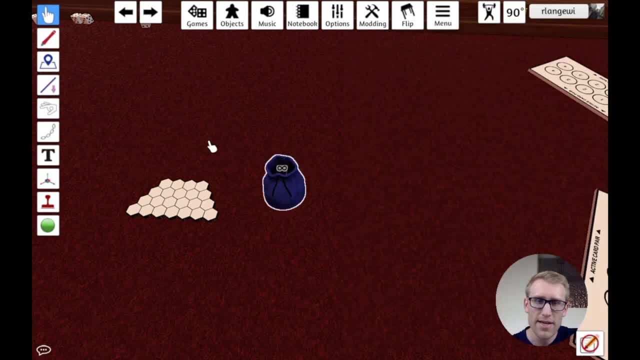 Infinite Bag And basically this is useful. So here I. I accidentally put my card, my deck of cards in the infinite bag. That's actually kind of funny. So what an infinite bag does is it shows here what, what component has been placed in it. 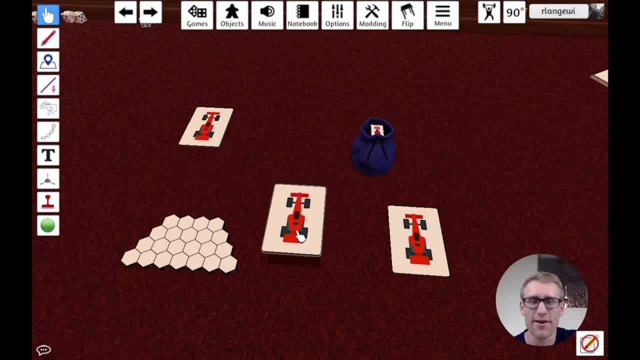 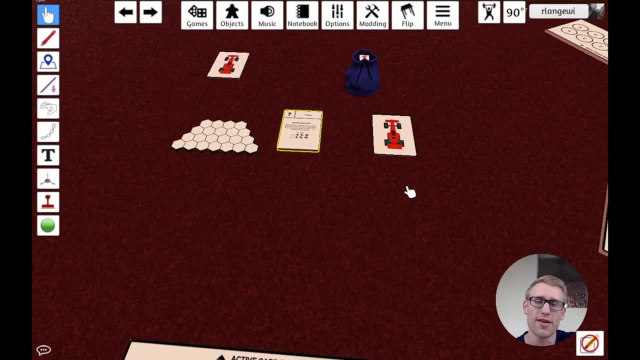 And then, whenever anybody draws out of that, they're going to get that component, which in this case is a set of eight cards, which is kind of a funny thing that I did there. But more commonly you could use that for like. 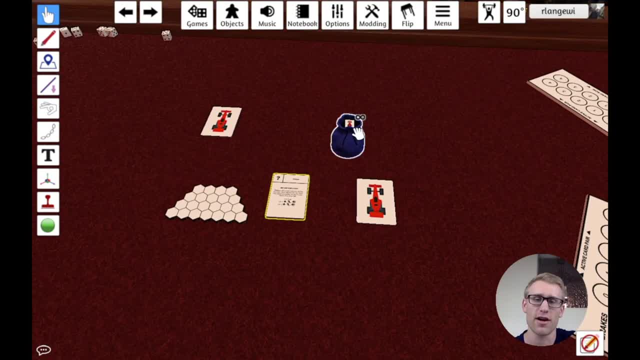 you know coins or some component that players are going to be like taking and returning, and you just need a bunch of them. If you don't have any specific restrictions on how many there are, you can just do that here. So suppose you got your game all set up here. 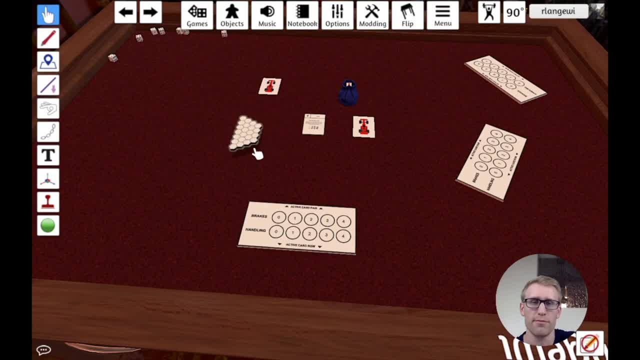 So you know I got these in. this is like the worst looking game of all time, but I would kind of set it up in what would be kind of the starting state for the game And then I wouldn't. I would want to save the mod in that state. 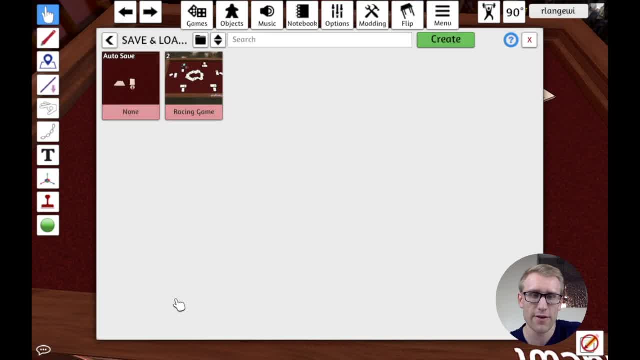 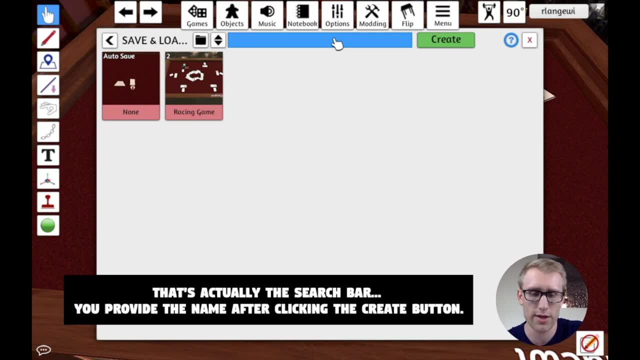 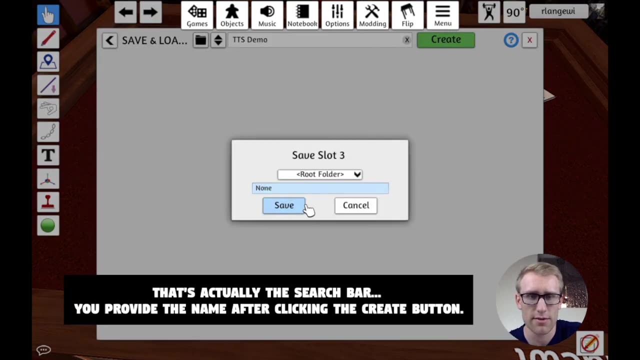 So that's where I'm going to go up to games here and go to the save and load section And by typing up in here I can create a new save file. So I'm going to say tabletop simulator demo and create save slot. 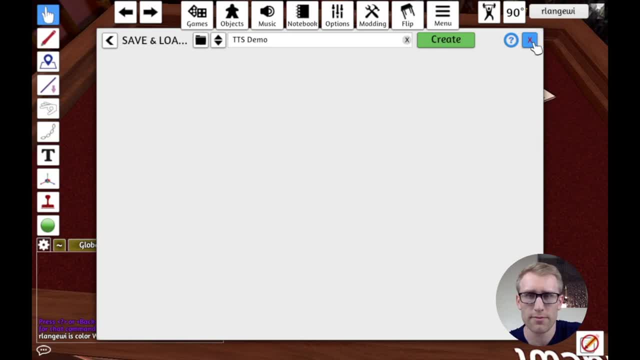 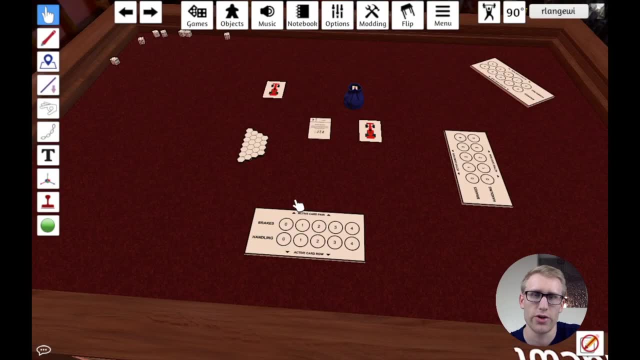 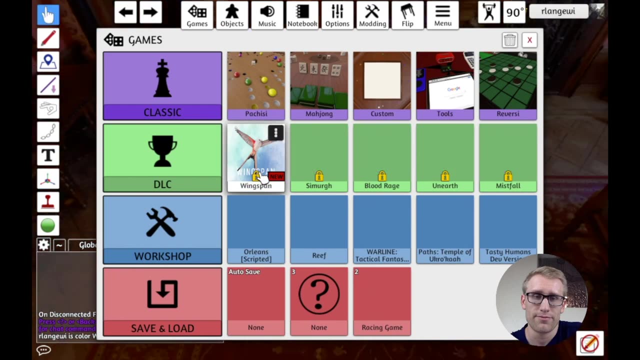 Sure. So if we go back here and, let's say, we go back to the main menu, are you sure? I'm very sure So, later when you come back into tabletop simulator and you go through that same process of going create in single player, 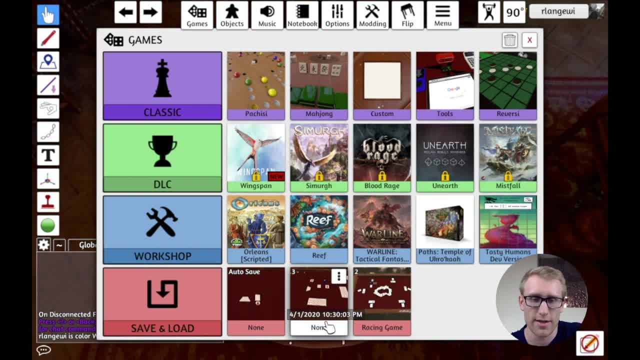 you can now see- and actually I guess I named it none instead of what I meant there. You can see this is now in the save spot. It also always auto saves whatever you were last doing in tabletop simulator. So I can now open this up and load it. 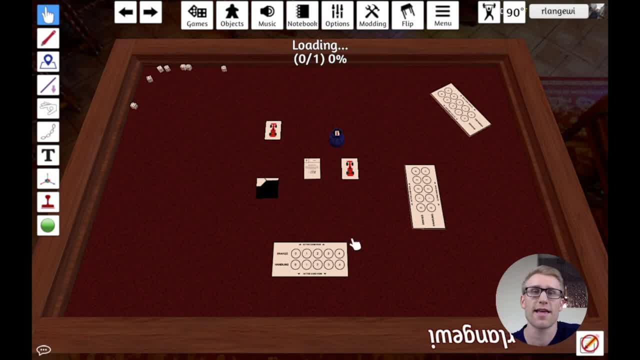 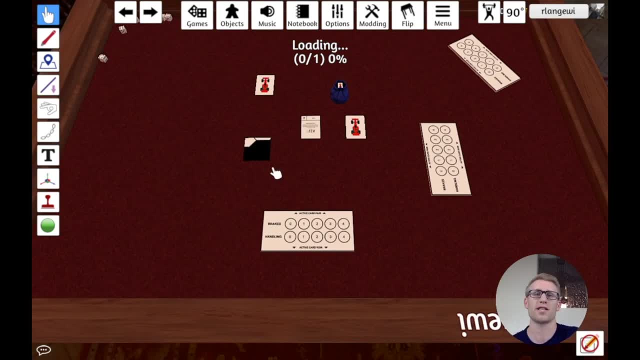 And it's going to be exactly in the state that it was when I when I saved it, And so this is very useful for you: get your game set up how you want it to be: at the beginning of a play test And whenever you want to start it. 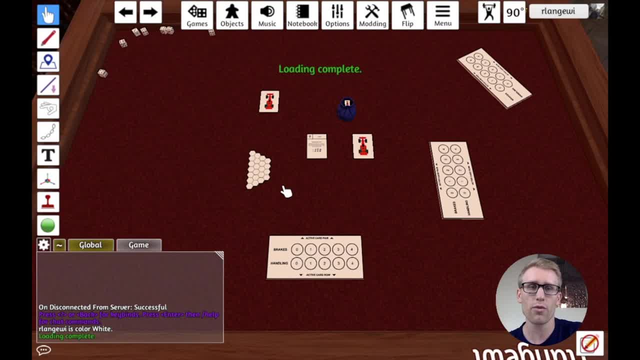 you just load the module and it's ready to go. You can end up learning how to then upload that module to the steam workshop and making it accessible for other people to download. You wouldn't need to do that to be able to play the mod with someone else. 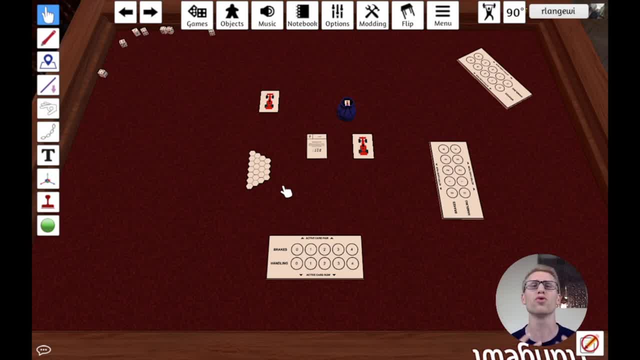 So, if you wanted to run a play test with some remote people, as long as you load the mod yourself and have other people join your server, as long as you've uploaded all your assets to be in the cloud instead of being locally on your computer. 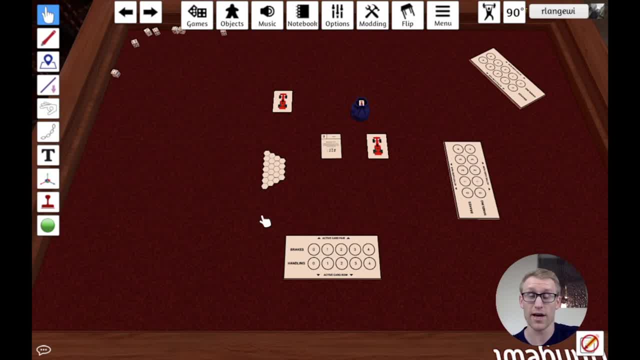 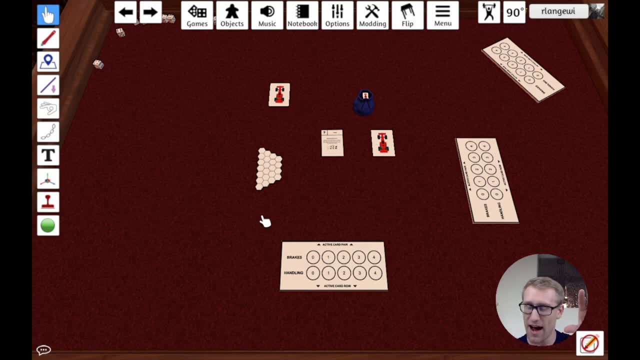 you should be able to play it with them. Fine, I don't want to get away from myself here. So those are just the basics of kind of what you might expect to be doing in tabletop simulator, And I want to just ask you. 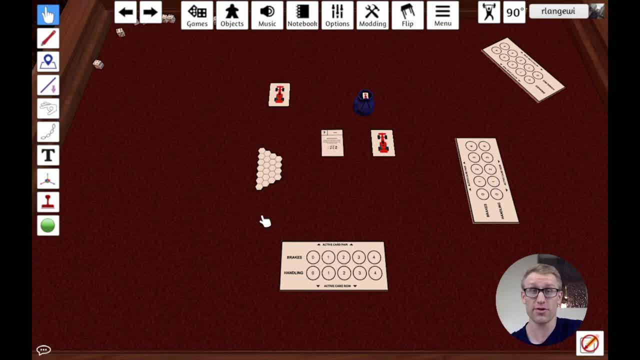 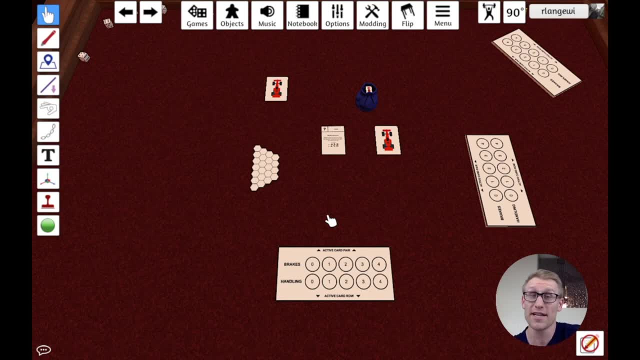 what would you like to see future videos on? Like I said, I'm not an expert in tabletop simulator- I've used it enough to feel comfortable in it- but I definitely would like to put out some more content of videos that might be helpful for people. 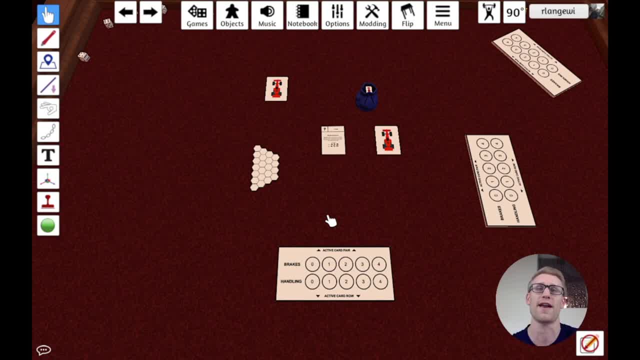 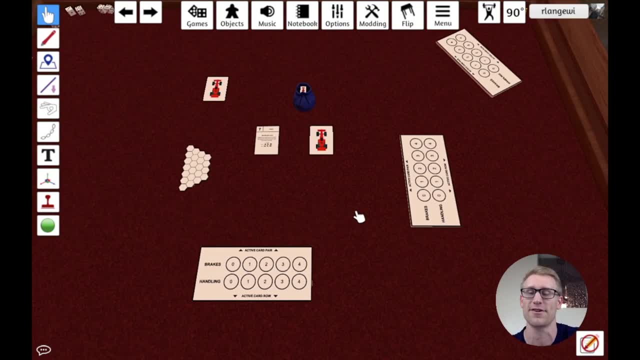 or even just learn some new skills myself and learn it well enough that I feel like I could teach it through a video. So let me know down in the comments. I'd appreciate it. Hopefully this was somewhat helpful. Like I said, there's lots of other good resources out there. 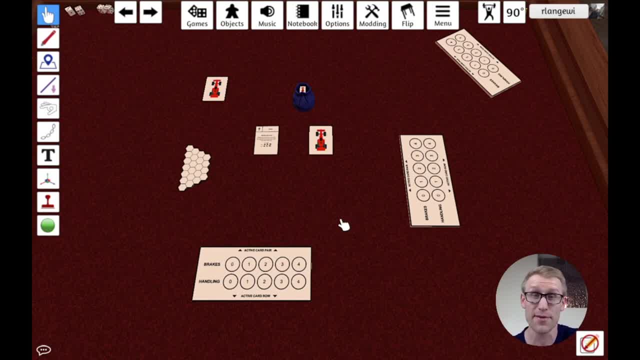 so be sure to check them out in the description. If you're interested in seeing more content like this, consider subscribing to the channel and I will see you in the next video.